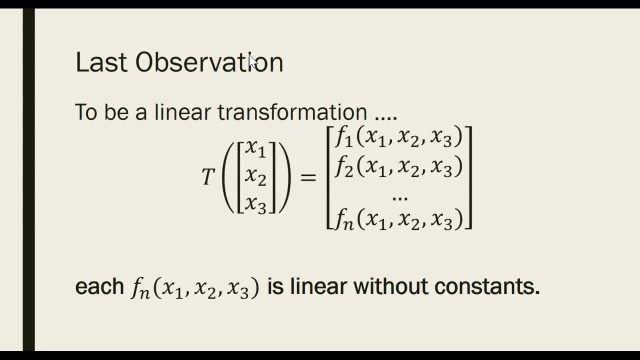 So what we're going to look at is is how to rewrite these. Now, if you remember from the last section, we said in order for a linear transformation to exist, we're going to have our input be a vector. Now, I chose a vector from R3 here, but it could be a vector from R2 or R4 or wherever. So just because it has three entries, I don't think they always have to have three entries, obviously. 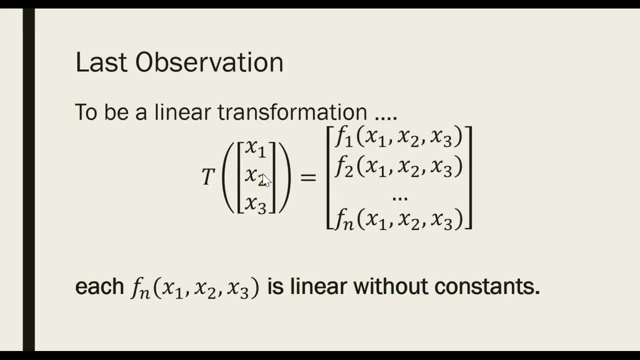 So we took a vector, our input vector, and our output vector has to have each entry as a function of variables from our input vector And that function, each of these, has to be linear and without constants, So linear, and then we can't have like a plus five constant at the end or anything. 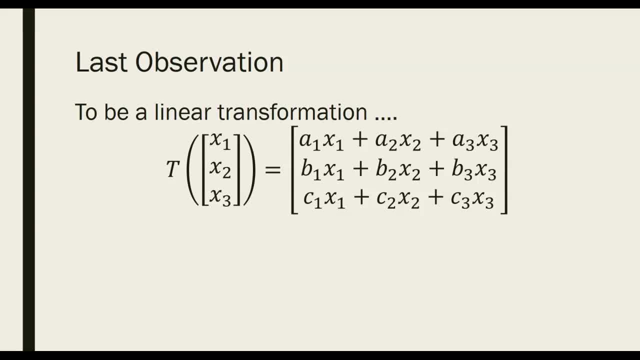 So it's going to have to look like this. Now I chose A's, B's and C's, but you could choose any letters you want. So if our input is a three-dimensional vector and our output is a three-dimensional vector, then this is what it's going to have to look like. 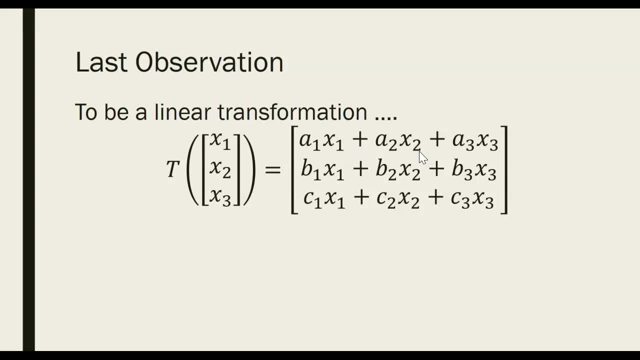 Okay, we're going to have x1, x2, x3.. So, in essence, a linear combination of x1, x2, x3.. So x1, x2, x3 has numbers. A linear combination of x1, x2, x3 has numbers in our second spot and a linear combination of x1, x2, x3 in our third spot. 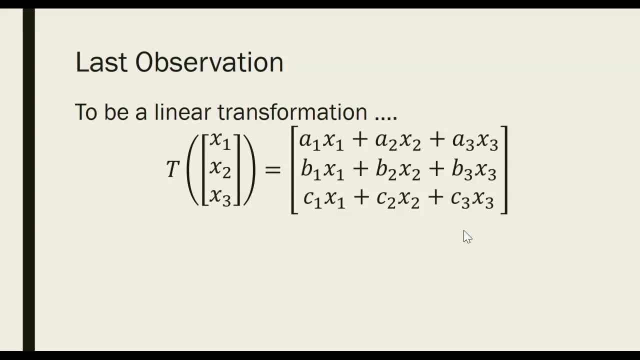 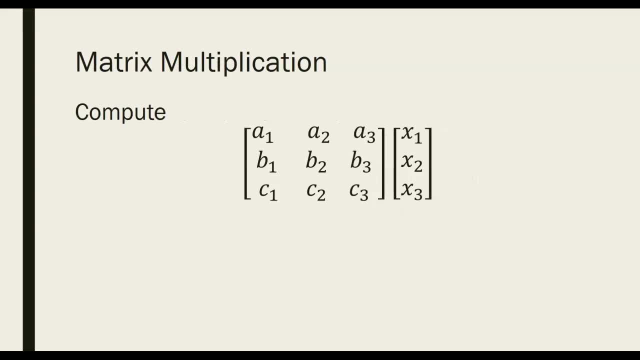 Again, no variables or, excuse me, no constant numbers other than the coefficients. Now I want you to think about what the resulting matrix would be if I took A1.. A1, A2, A3, and B1, B2, B3,, C1, C2, C3, and multiplied it by this three-dimensional vector. 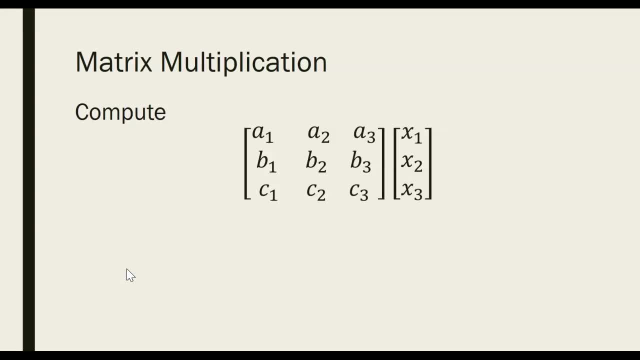 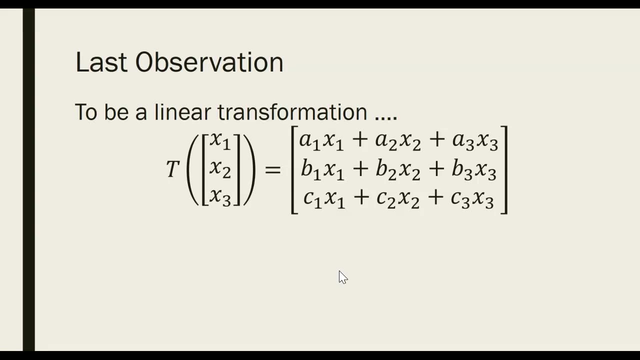 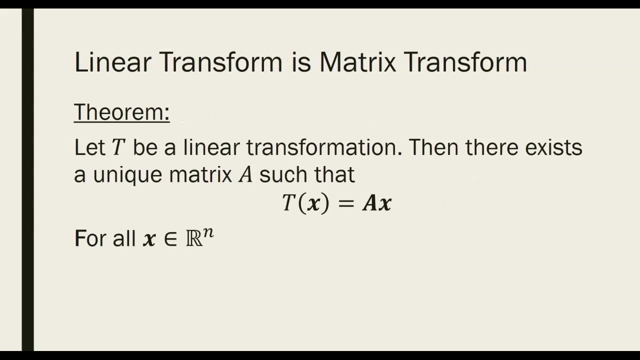 In fact, I want you to just push pause on the video and go ahead and do that yourself, All right, so hopefully you went ahead and did that. Oh, excuse me, I did the multiplication, sorry- of this matrix times this vector. 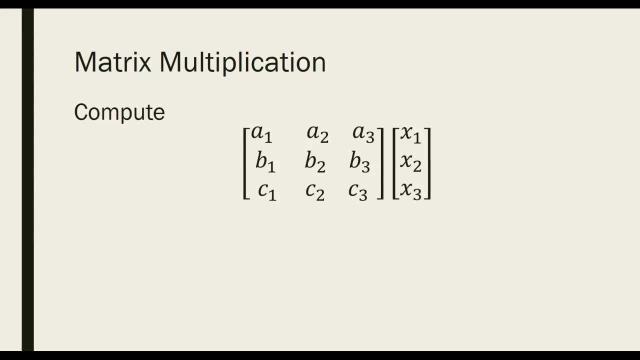 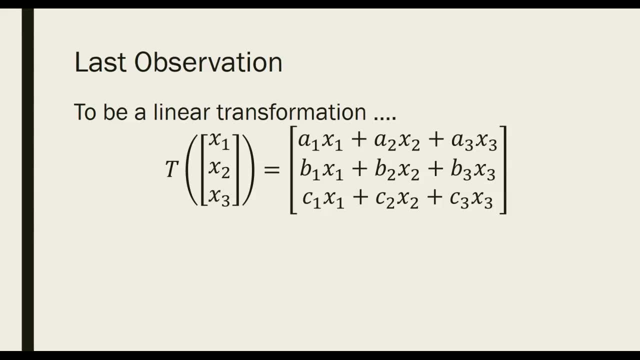 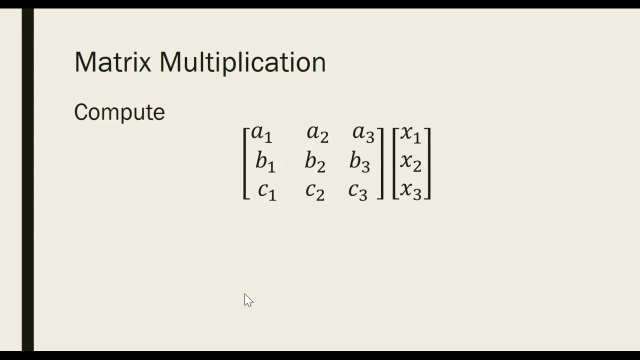 If you do that, you see that the output is going to be exactly the same as the linear transformation I wrote in that previous slide. Okay, so this linear transformation has the same output as this matrix multiplication. I just want to go show you how to do that real quick. 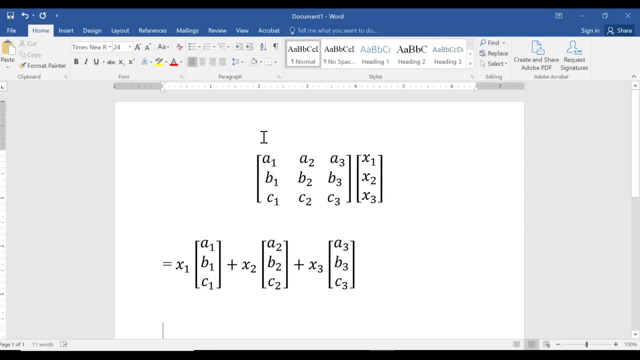 If you have forgotten. so what we do is we take this first column. we'd write that as a vector times x1.. This second column: we'd write that as a vector times x2.. Third column: we'd write that as a vector times x3.. 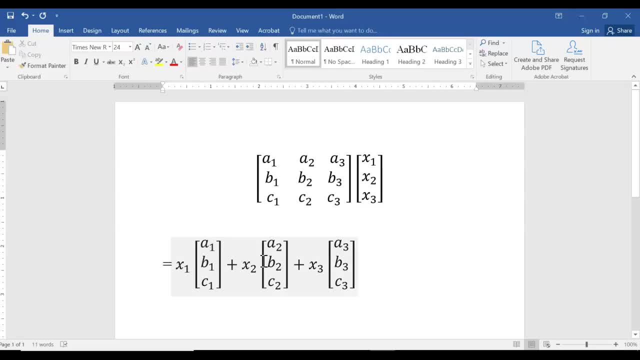 And then, when you add this up, this would be A1 times x1 plus A2 times x2, plus A3 times x3. That would be your first entry: B1 times x1 plus B2 times x3. B2 times x2 plus B3 times x3 would be your second entry. 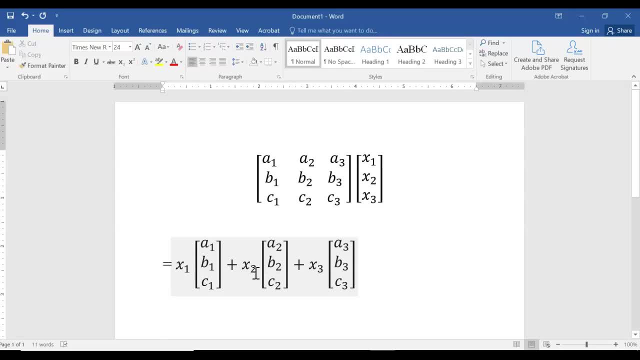 And then again: C1 times x1, C2 times x2, C3 times x3 would be your third entry. All right, so you'd get the matrix again. That was the output matrix of an arbitrary linear transformation. Okay, from again that linear transformation. 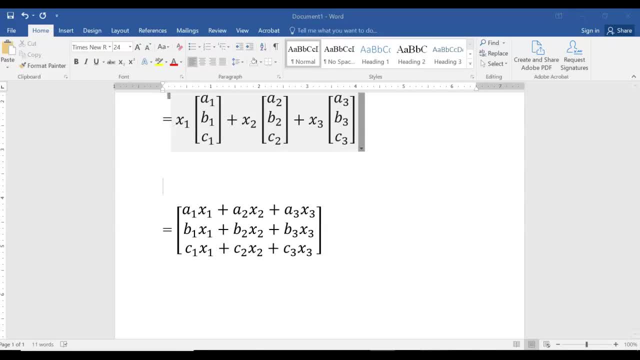 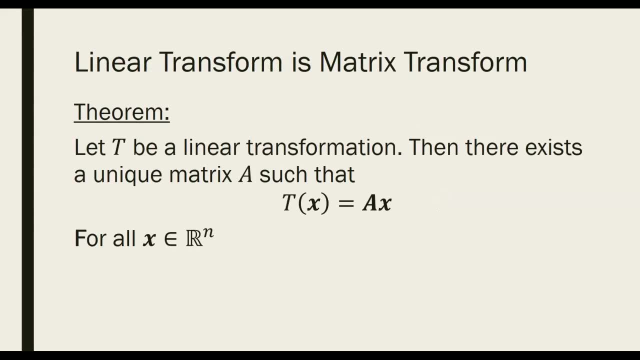 The linear transformation was from R3 to R3.. But what this shows you is that every linear transformation is actually can be thought of as a matrix transformation. In other words, if we're from Rn to Rm and T is a transformation. 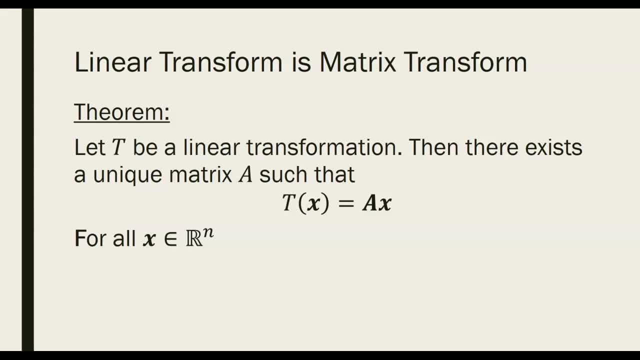 it is some matrix that would give you the same result as the transformation on any arbitrary vectors. So, in other words, the transformation times an arbitrary vector is going to give you the exact same thing as the matrix multiplied times the vector. So for every linear transformation, for every linear transformation, 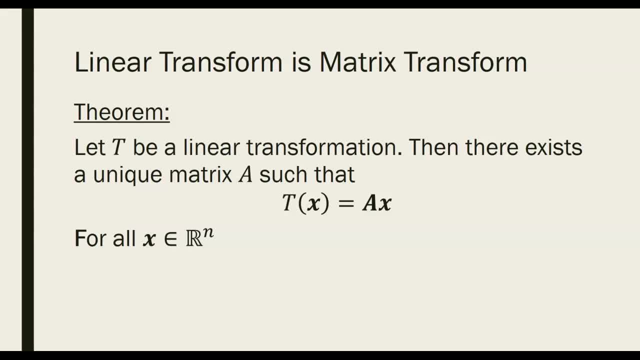 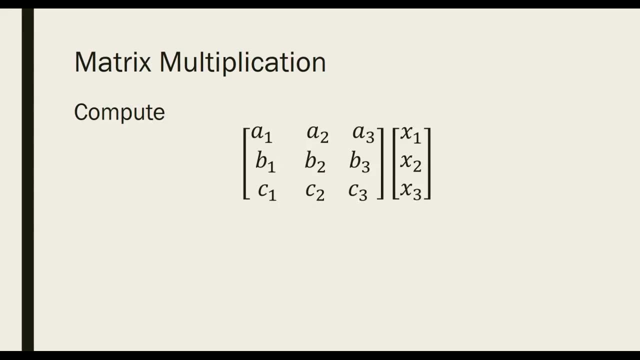 there is a unique matrix that the linear transformation applied to any vector is going to give you the same result as that matrix multiplied times the vector. Okay, By the way, the proof is basically just this. We just say: well, how big of a matrix do you want? from R what to R what? 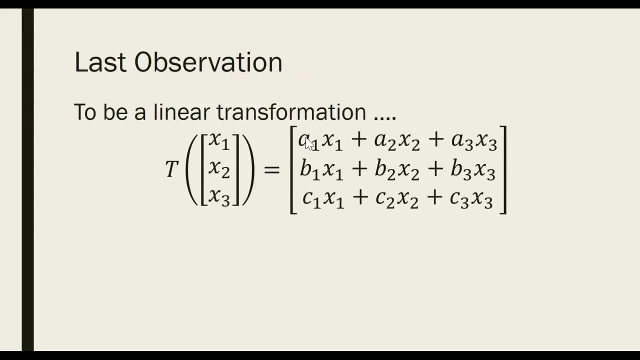 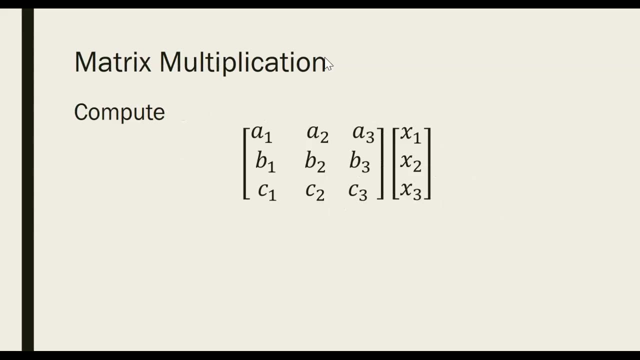 And then say: well, because each entry And our output vector is a linear function without a constant. We can create that by taking the linear functions, as you know, basically this: a1, a2, a3, this row times our vector. 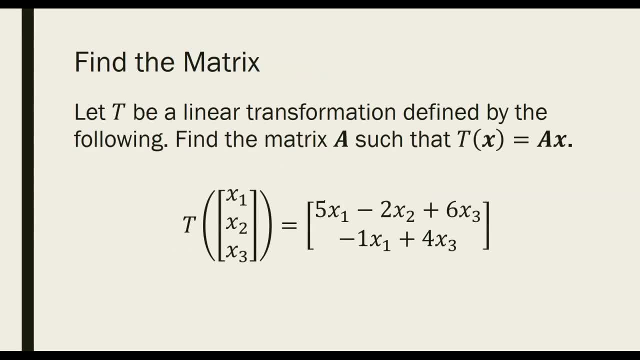 Hopefully that makes sense. Okay, So I want you to do this. Let's try it, Let's try it, Let's try it. Let's try to find a matrix such that, if you have this linear transformation that's defined here, such that that transformation times any vector, is a times that vector. 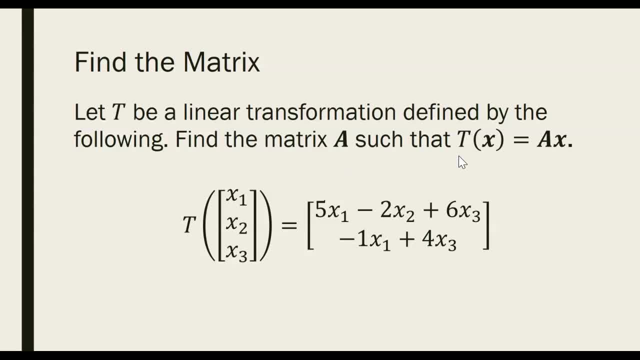 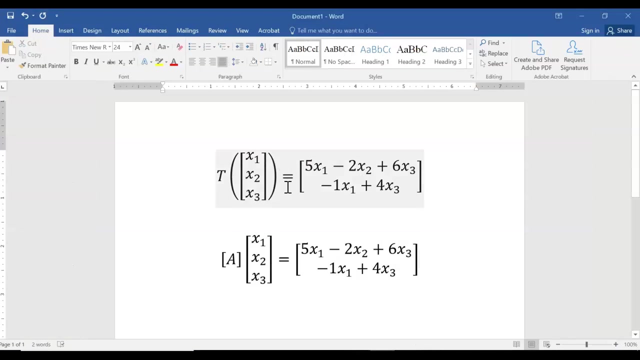 So try to find the matrix that's associated with this linear transformation. Push pause on the video and see if you can go Go ahead and do that, All right. So hopefully you did that. Basic idea here is that we want to create a matrix that has the same output. 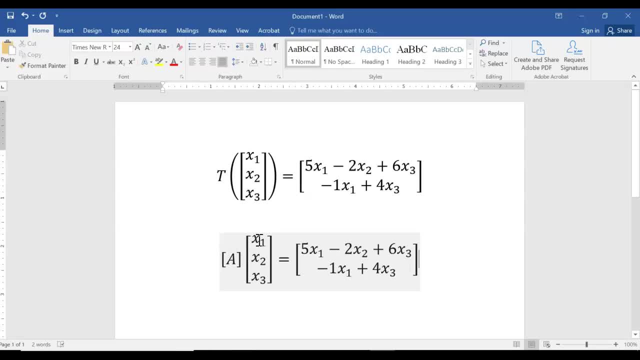 So I'm thinking of a matrix A which, when you multiply it, times the vector x1, x2, x3 gives us this: Now, if we remember from last time, what's going to happen is that x1 is going to have to be multiplied times the first column, x2 is going to have to be multiplied by the second column, x3 is going to have to be multiplied by the third column. 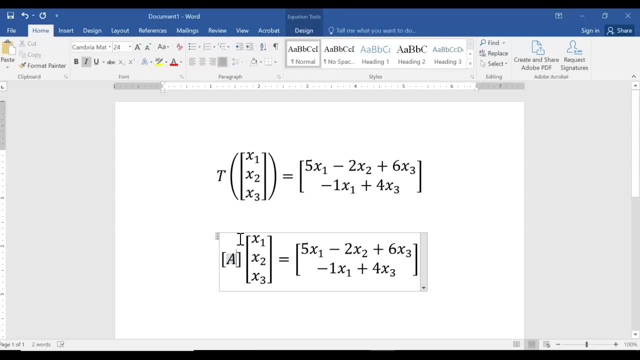 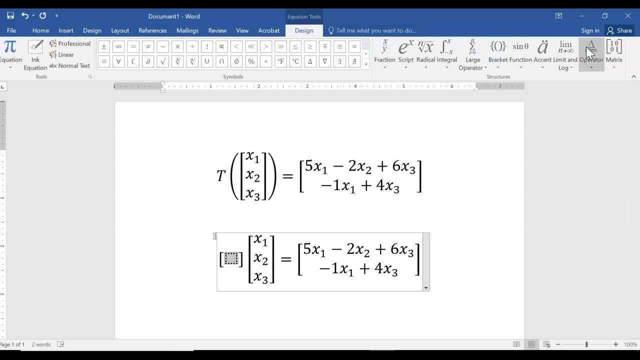 That tells me that there's going to be three columns in our matrix. because I need to multiply by x1, x2, x3. And because my output vector has just two rows, I know my matrix A is going to be two rows. 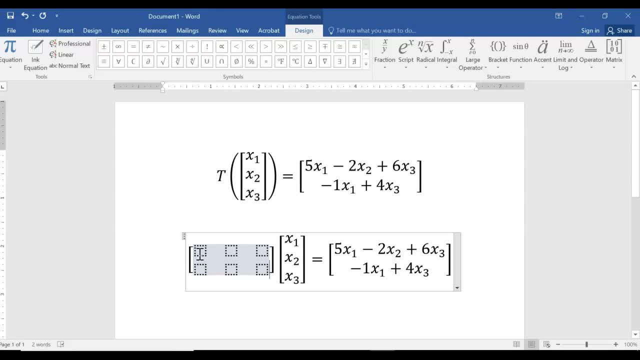 x1, x2, x3.. Two rows and three columns. It's going to be this big, All right. Now I know that x1 is going to have to be multiplied by the first column, So all I have to do is go over here and say: okay, x1 is multiplied by 5 in the first row and negative 1 in the second row. 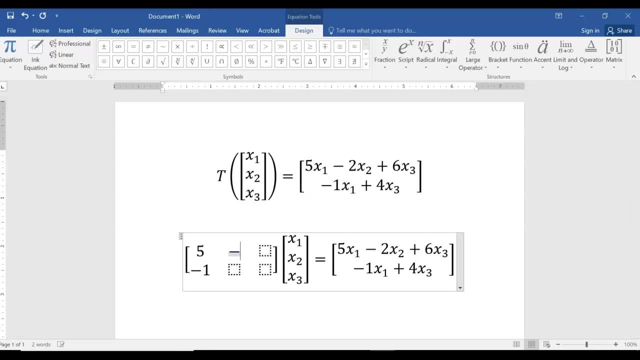 x2., x2., x2., x2. x2.. multiplied by a negative 2 in the first row. In the second row there's no x2, so we'll just label that as 0.. And then, lastly, we have a 6 and a 4 as my coefficients of x3. that are in the first. 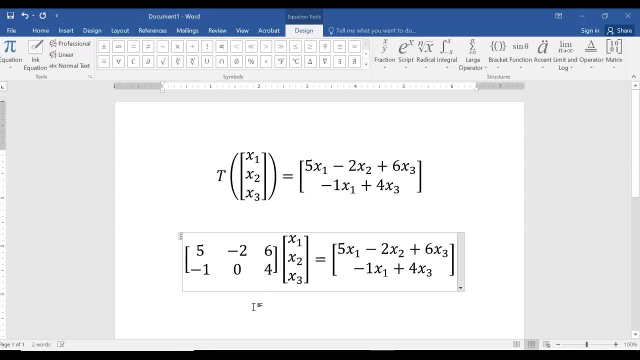 and second row respectively. So the matrix A that I'm looking for. the matrix that I'm looking for is 5, negative 2, 6, negative 1, 0, 4.. Okay, And it's a pretty straightforward process. 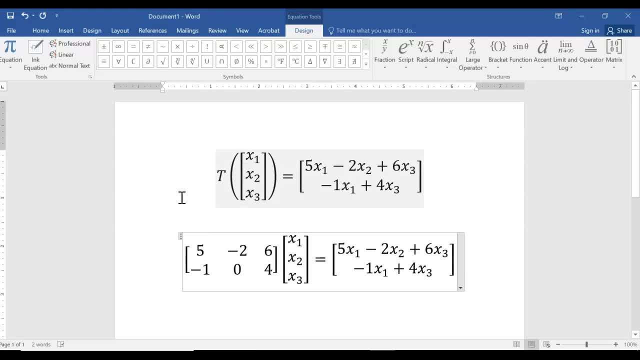 Anytime you have this, all you have to do is again: first column is going to be your x1s. second column is going to be your x2s. third column is going to be your x3s, and so on and so forth. 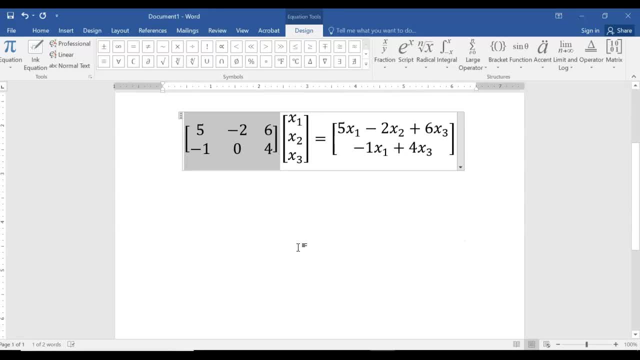 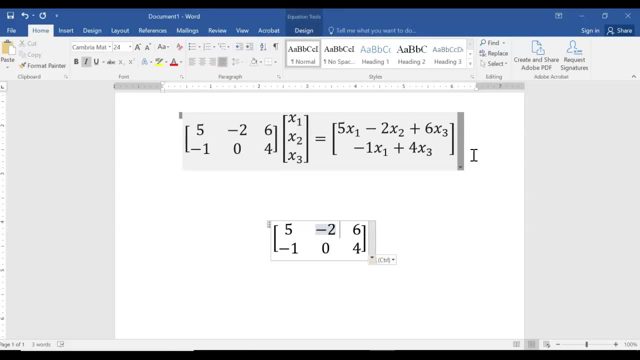 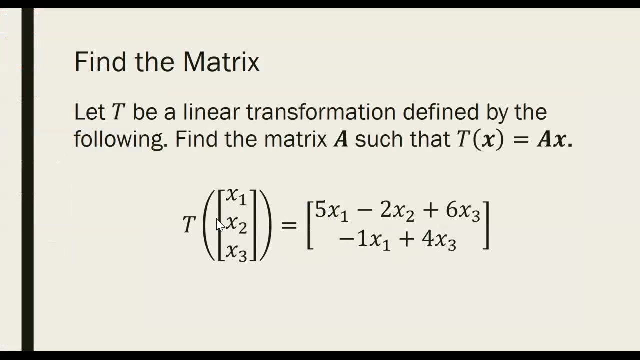 Okay, So the matrix that we wanted- Oops, let me do this. We would say that matrix A, the one we were looking for, must have been that All right. So that's the big idea, And if you have a transformation that's defined this way, 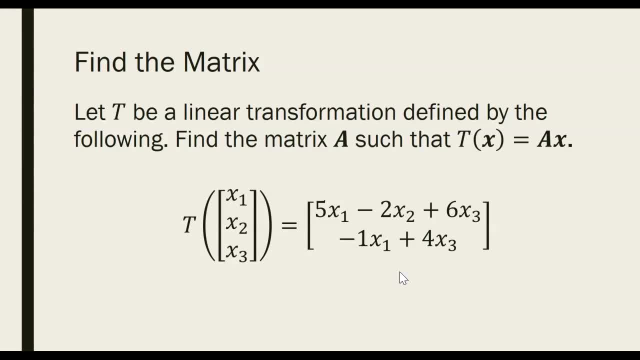 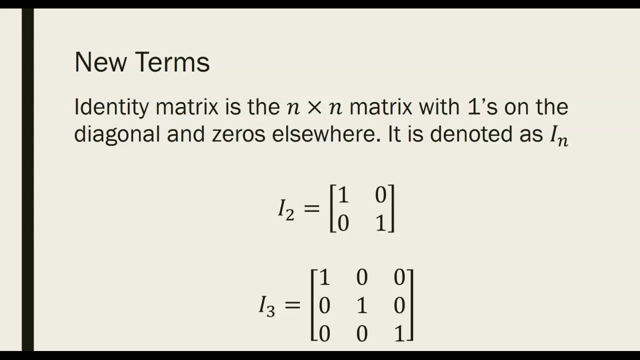 then it's a pretty nice, easy process to actually find the matrix that defines that, That linear transformation, or the- I should say the matrix which is associated with that transformation. Now we're going to look at another way to talk about finding the matrix. 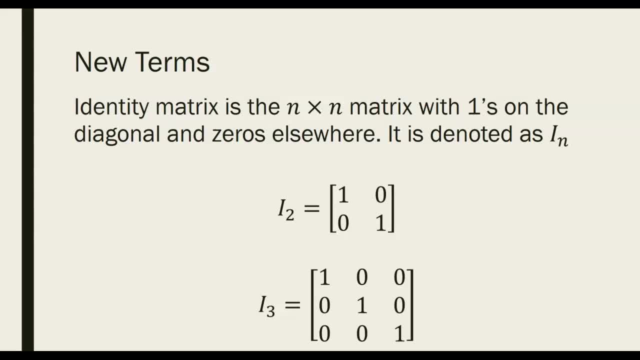 but that other way is going to need some terminology. So what I'm going to do is I'm going to talk about what's called the identity matrix. All right, The identity, the identity matrix, is going to be an n-by-n matrix. We call that a square matrix. when the 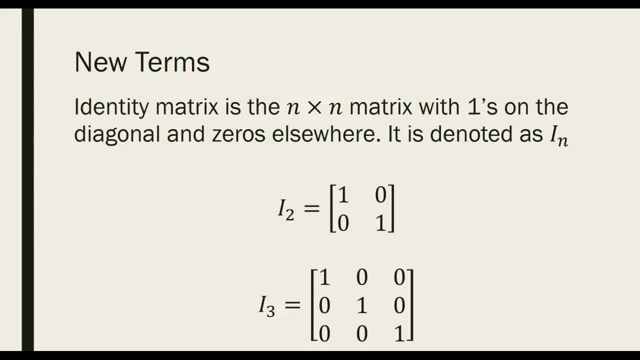 number of rows and columns are the same, So it's going to be a square matrix n-by-n, with 1s on the diagonal- technically the main diagonal- and 0s elsewhere. Okay, So if we have 1s on the upper left, working ourselves to the lower right, and it's a square. 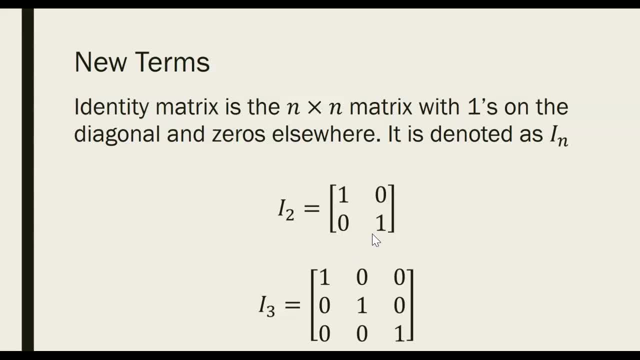 matrix. that's called the identity matrix. We saw a lot of these when we put things into row-reduced echelon form. Okay, I don't think I used the term identity matrix, but that's what it was. So when we put things into row-reduced echelon form, we have the identity matrix. 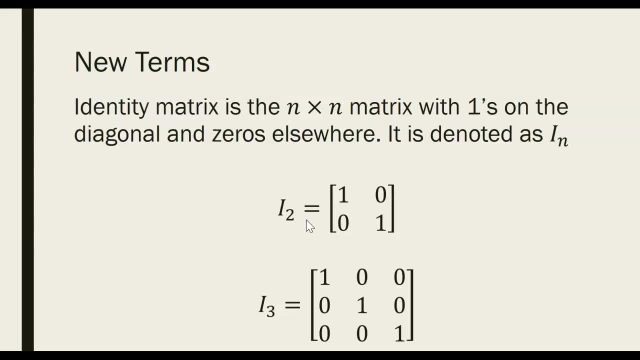 Now the subscript. here the n is just how big it is. So i sub 2 is a 2-by-2. identity matrix. i sub 3 is a 3-by-3 identity matrix We could have i sub 5. That would. 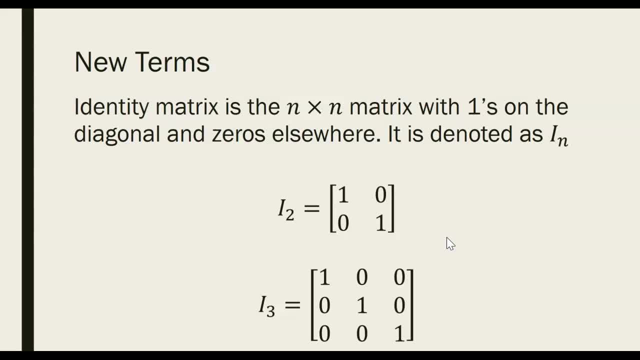 be a 5-by-5 identity matrix. Now, the identity matrix itself isn't the most important part of this chapter or, excuse me, of this section. The identity matrix is useful in that we want to look at the columns. All right, These are really nice columns. 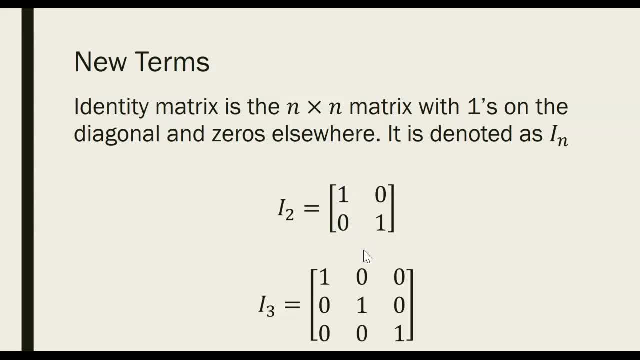 We have a 1 in a certain spot and 0s elsewhere. A 1 in a certain spot, 0s elsewhere. Those types of rows and columns are really nice to deal with when we're talking about row-reduced echelon form, but they're also really nice to deal with when we're talking 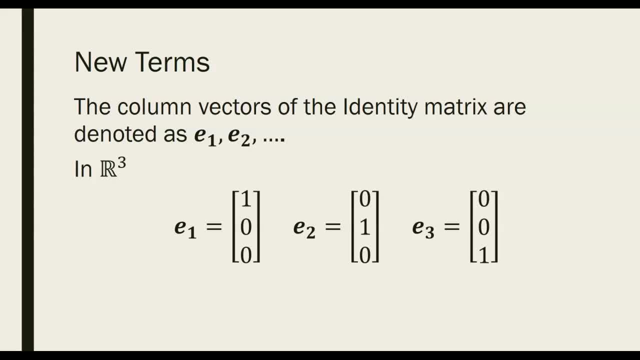 about multiplying matrices. All right, So we're going to create what we call E1, E2, E3, E4, etc. etc. etc. And basically those are just the column vectors in our identity matrix. Okay, So E2 stands for having a 1 in the second entry and 0s elsewhere. E3: 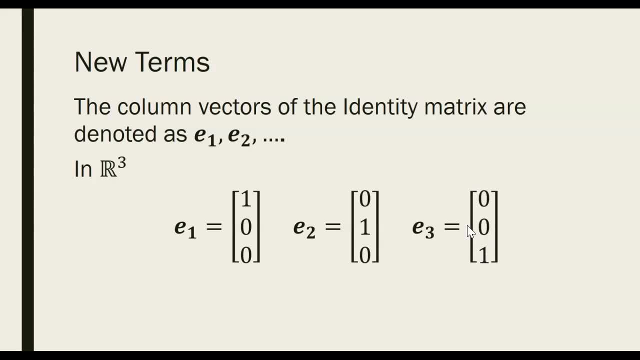 stands for having a 1 in the third entry and 0s elsewhere. E1 has a 1 in the second entry and 0s elsewhere. E16 would have a 1 in the sixteenth entry and 0s elsewhere. 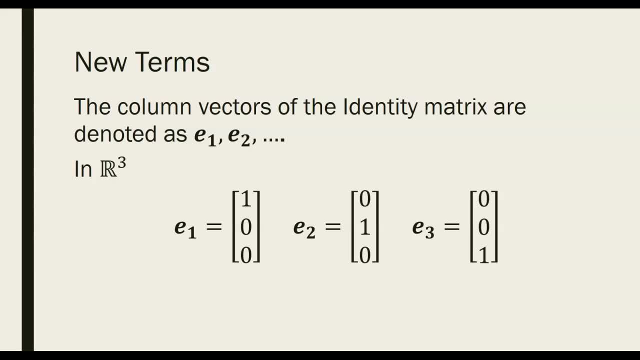 if we were in a big enough dimension where E16 existed, All right. So you can see that in R3, if you only have three dimensions, then there's only going to be three Es. If we were in R4, there would be four Es. 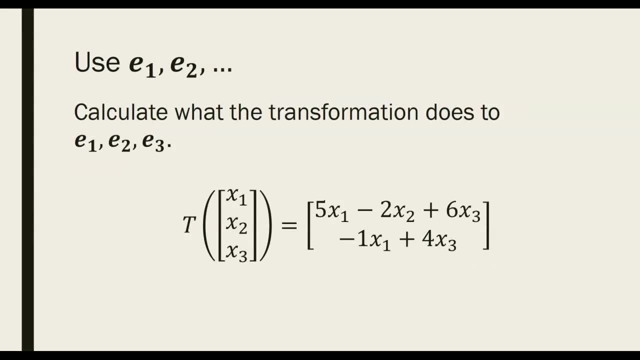 Pretty straightforward, Okay. Now what we can do, or one way to think about the transformations, is ask: what does the transformation do to E1,, E2, E3?? What does it do to those column vectors in our identity matrix? Okay, 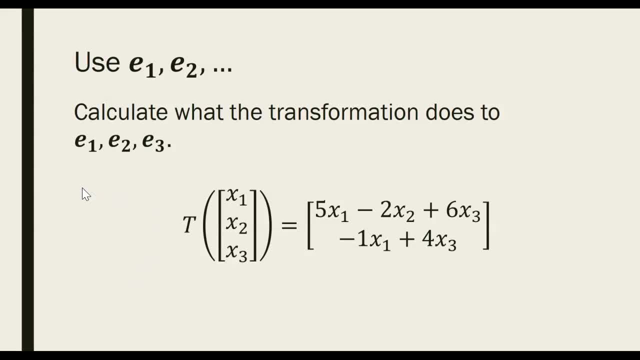 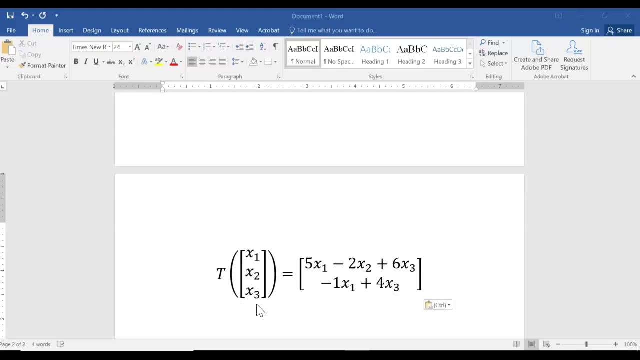 So let's calculate what those things are and then show how that's related to the matrix we found earlier. So just as a reminder, our transformation is here, and last time we did this we kind of logically just said: oh yeah, these have to be the coefficients, and so on and so forth. 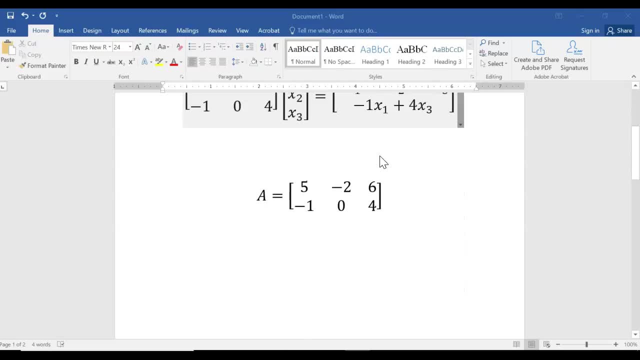 And that's how we found A. But I want you to notice what's going to happen when we put in- oops, the vector 1, 0, 0.. Okay, Okay, Okay. Now I'm not going to write this every time, but I will the first time. 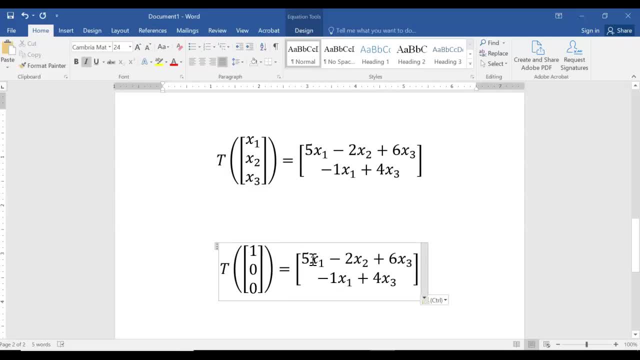 Think about what's going to happen to our output vector. Everywhere I see an x1, it's going to be replaced with a 1 that I'm multiplying. Every time I see an x2, it's going to be replaced with a 0.. 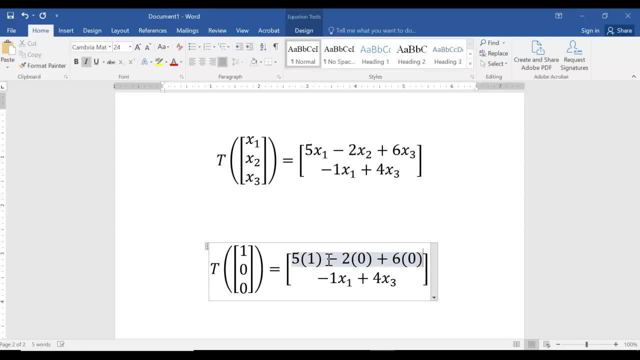 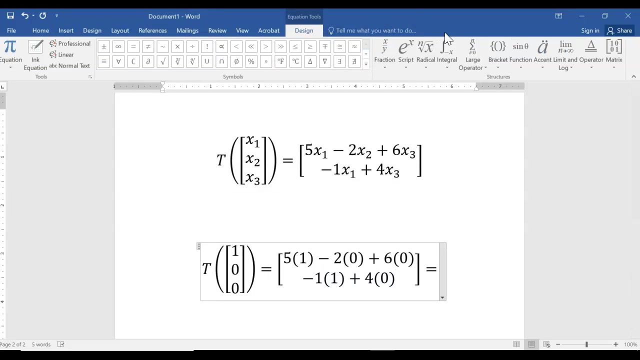 Every time I see an x3, it's going to be replaced with a 0. So, basically, what's going to happen is that the terms with the x2s and x3s are going to go away And, by inputting 1,, 0,, 0,, the only thing we have left are essentially just the coefficients. 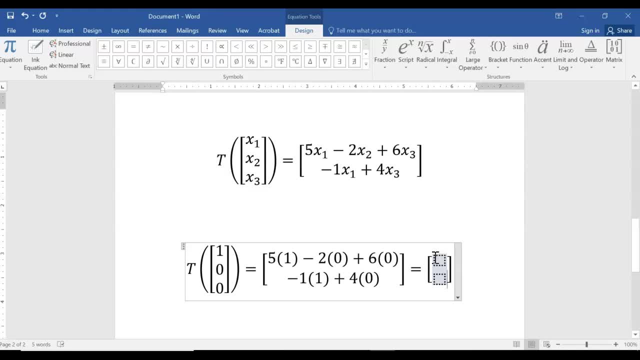 of the terms with the x1s. all right. So we basically are ending up with a 5, negative 1.. So what that tells me is that, Again, remember what matrix we had earlier. we found 5, negative. 1 was our first column. 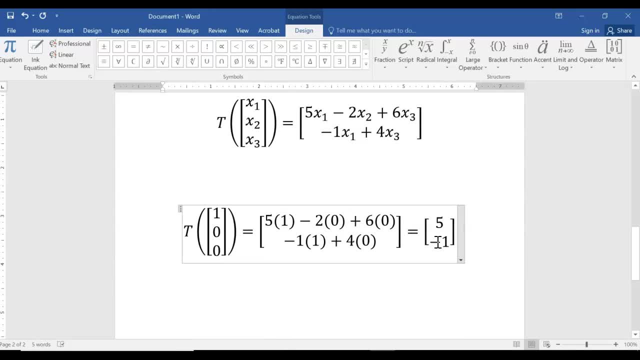 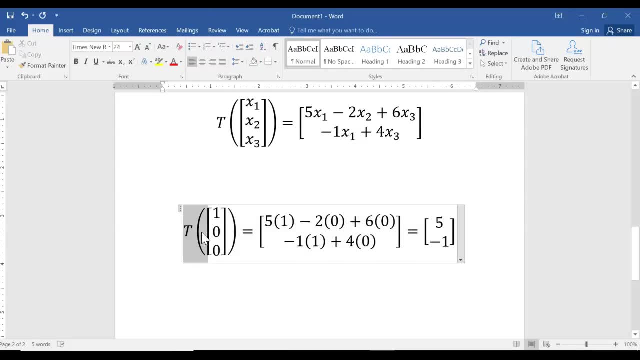 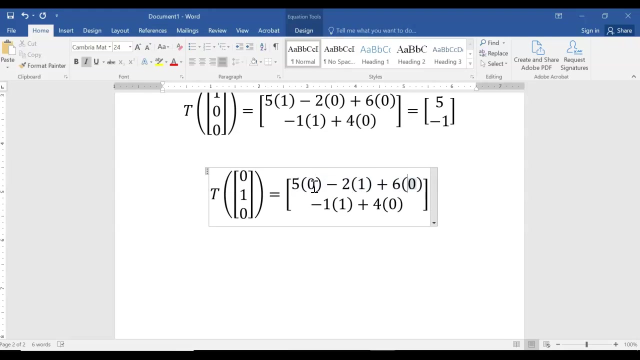 So if we input E1, we got the first column of our matrix. Now, I'm not going to do this long form every time, but it's pretty obvious that if we input E2. Scroll up, All that's going to be left- the terms with the x1 and the terms with the x3 are going. 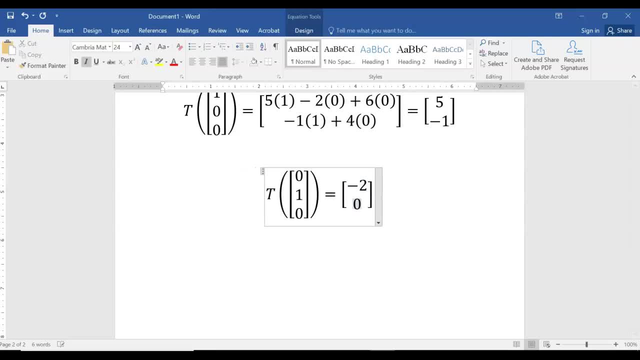 to go away. The only thing that will remain is the coefficients of the x1 and the terms with the x2.. So I'm going to do this long form every time And by inputting 1,, 0,, 0,, the only thing we have left are essentially just the coefficients. 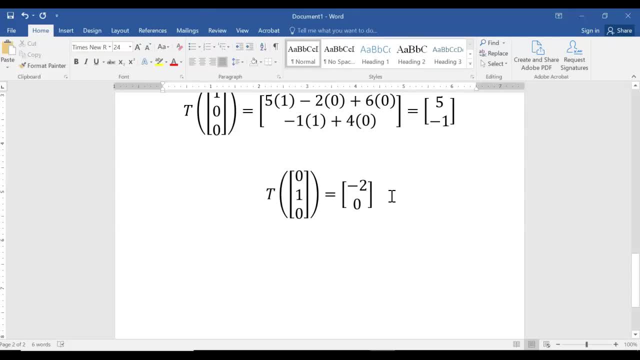 of the terms with the x1s and the terms with the x3s are going to go away, And so we get the second column in our matrix And without doing the calculations, you can imagine that when you plug in E3, you end. 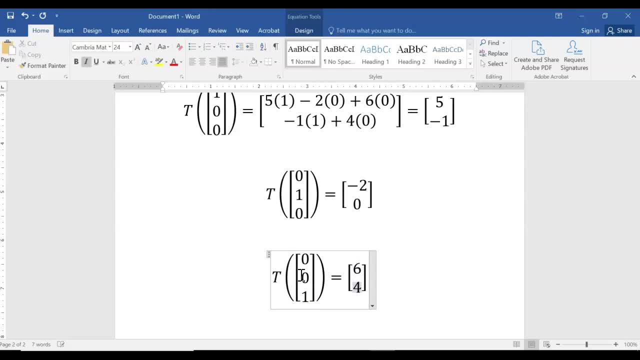 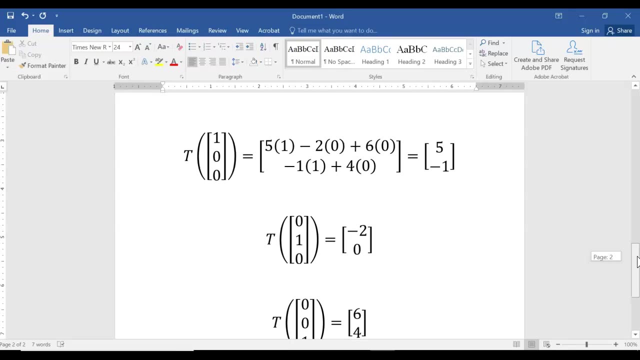 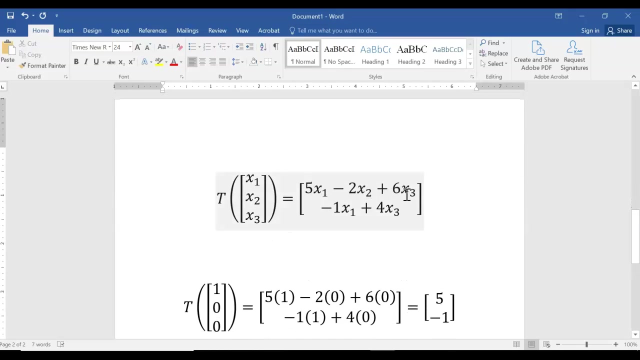 up with the third column of my matrix A. All right, Now you can see why that has to be the case, right? No matter what dimensional spaces we're in, this was not a fluke. Every time you're dealing with a linear combination. if you plug in one of the E's, let's say you. 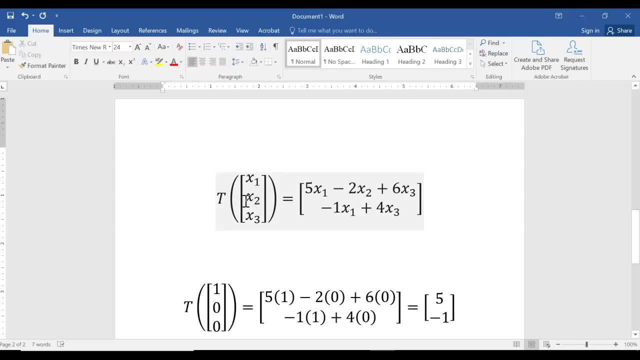 plugged in E2, it's going to give you all the coefficients of the x2 and none of the coefficients of x2.. If you plug in x1 or x3, if we were in a five dimensional space and you plugged in E4, you'd 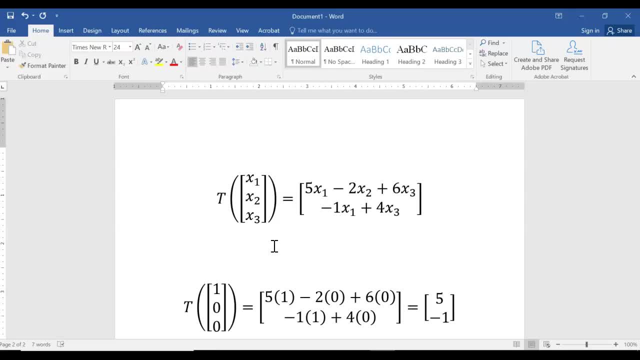 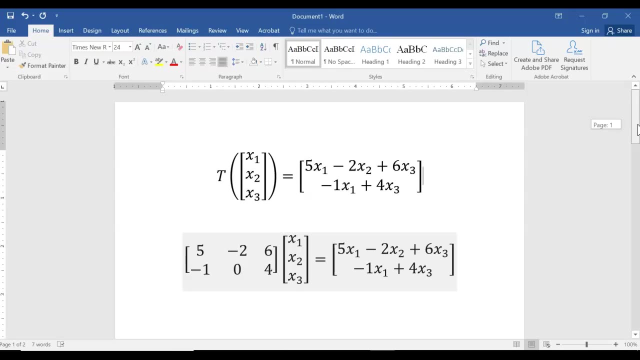 get all of the coefficients of the x4 in an arbitrary vector. So this tells us, if I don't have a transformation explicitly defined for me, if I know where the transformation sends- E1 and E2 and E3. And so on and so forth- I can, I can find a matrix that describes that transformation. 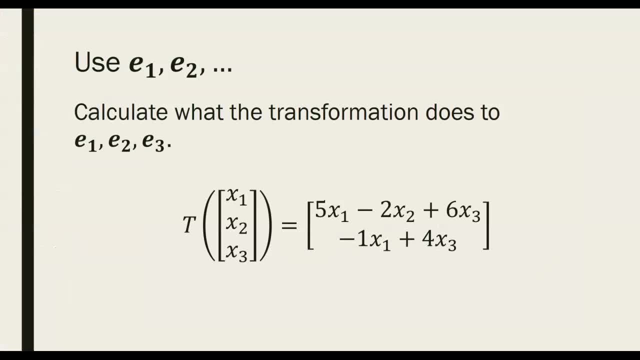 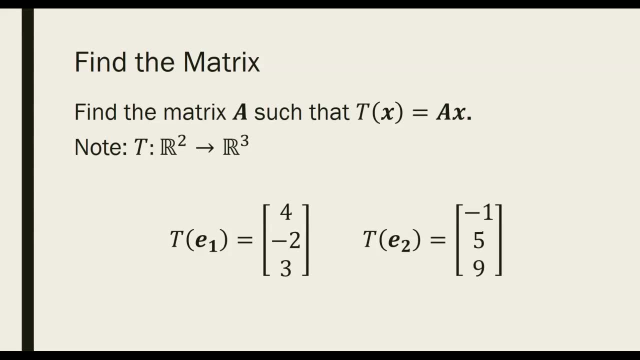 So that's what I want you to do. I want you to take this and figure out a matrix so that the transformation multiplied times a vector, Or the transformation of a vector, is the same as the matrix multiplied times the vector. Now, here's what I want you to note. 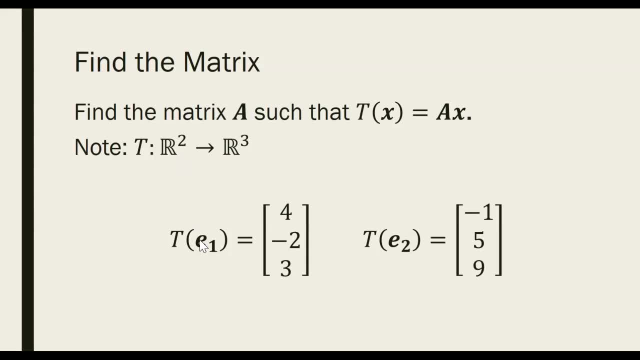 We're going to start in R2.. So we're going to start in R2.. We're going to have an E1 and an E2.. Again, think two by two identity matrix, And I'm going to get out a vector in R3.. 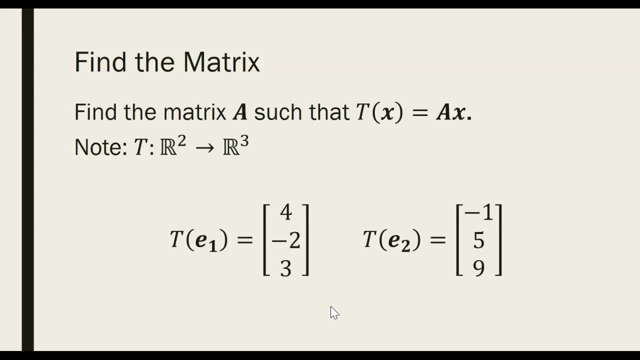 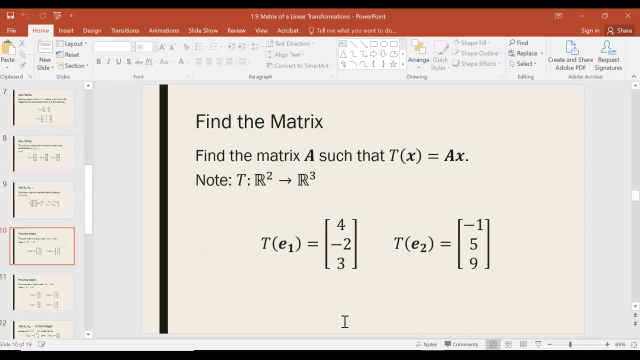 So you can see those two vectors there. All right, Push pause on the video And see if you can do that. This is not a hard or difficult situation. Again, once you get the hang of it, Let's go ahead and do this example. 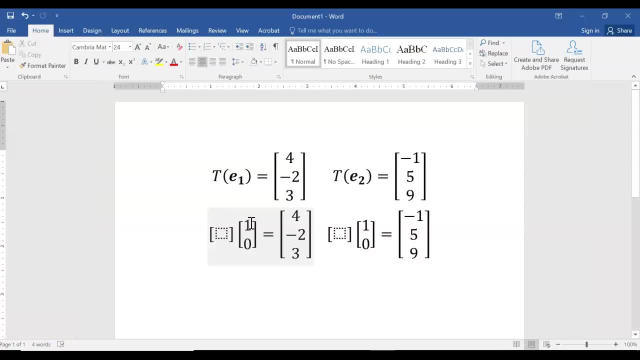 So basically I want a matrix that when I multiply times one zero, I get four negative two, three. Now This matrix times one zero is just going to pull off the first column. So in essence, that first column. Well, first off. 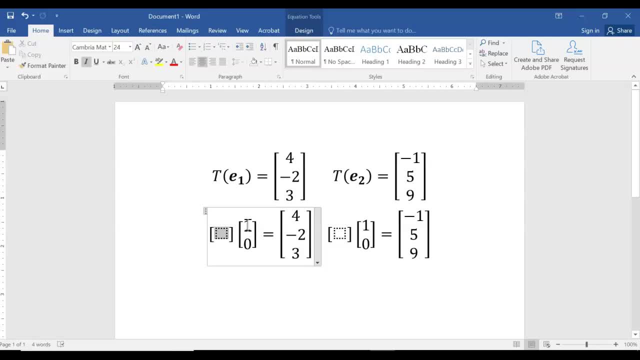 Notice: since we're going from R2.. Since we're multiplying by a vector from R2.. We're going to have two columns. And since we're getting in vectors from R3. Getting out vectors as output vectors from R3. We're going to have three rows. 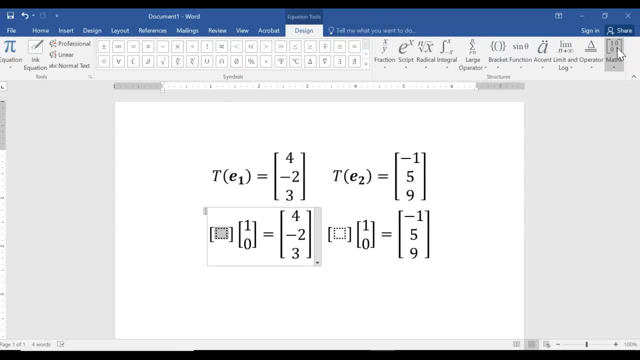 So when we create this, It's going to be a three by two matrix. When you multiply times one, zero, It's going to pull off the first column. So basically it just says my first column is going to be four negative two three. 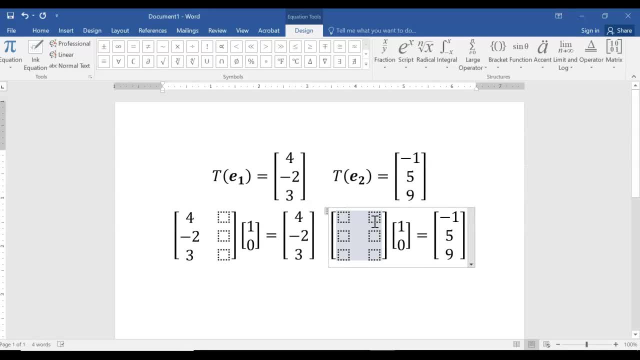 Same thing over here, But we're going to pull out our second column, So the second column Is going to be negative one. Oops, I'm sorry, Mistake, Mistook, that Put E1 instead of E2.. In my. 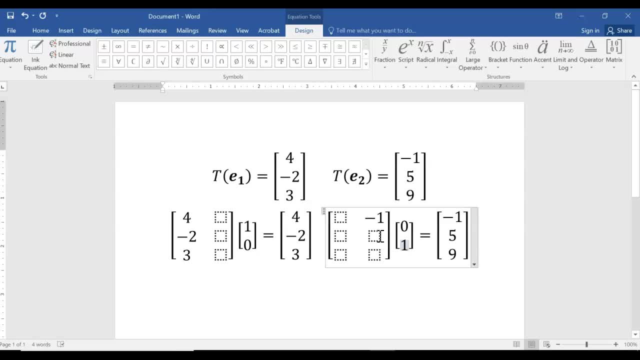 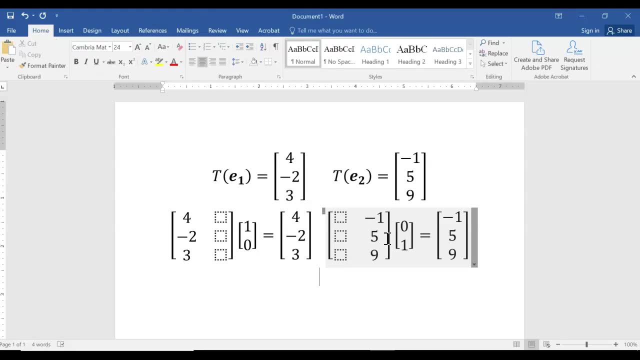 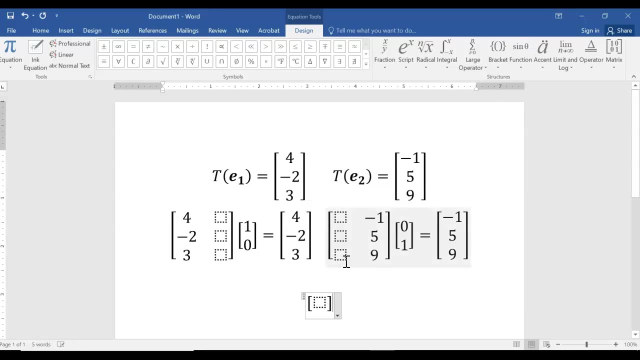 No, It's there. So Zero one. You pull off the second column When you multiply times E2.. So there you go. So it's pretty obvious that the matrix has to have the first column as four negative two, three. 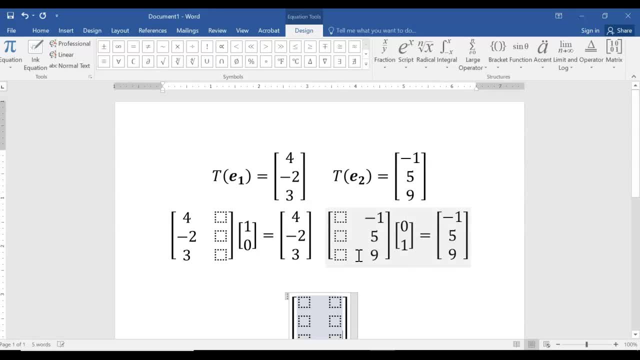 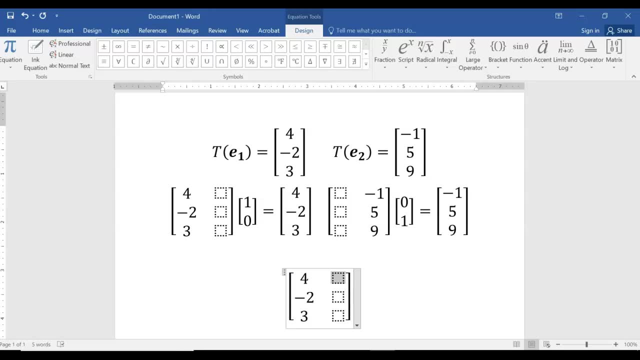 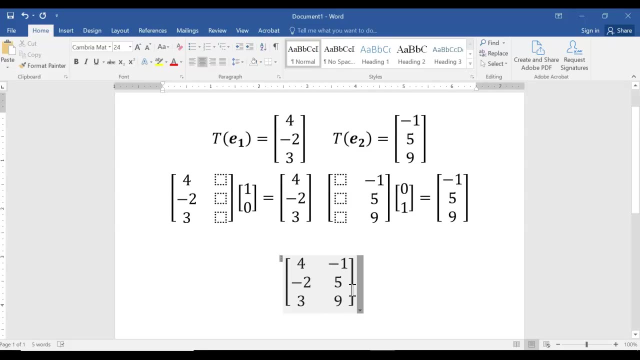 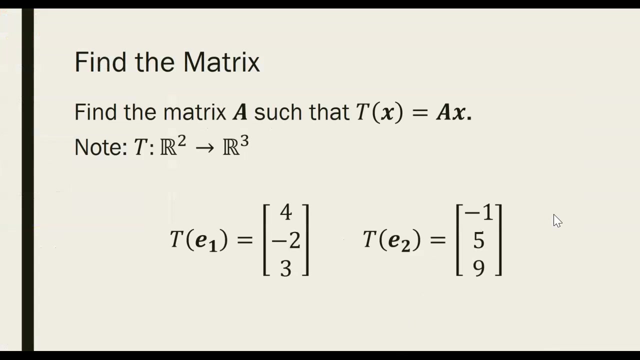 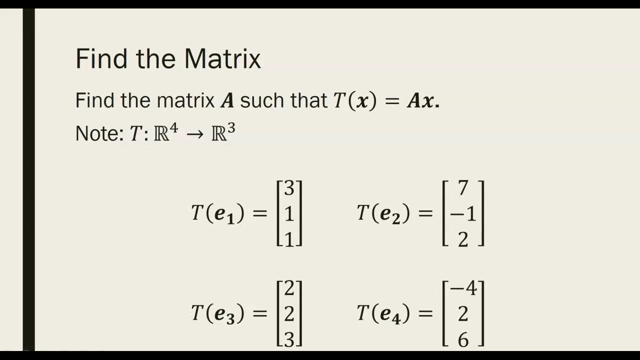 And the second column as Negative one Negative nine. And there we go. All right, So that's your matrix A. I want you to do the same thing For the next example. So push pause on the video And, hopefully. 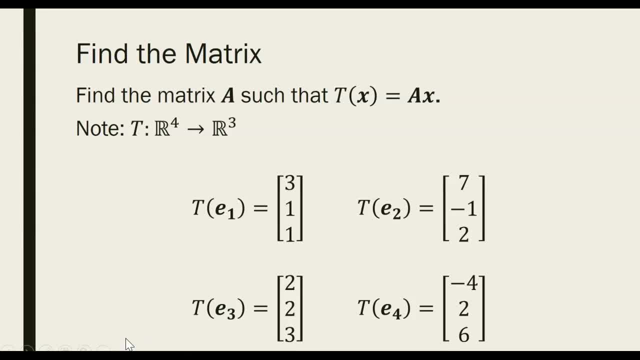 I'll move that slide just slightly down. There you go. So push pause on the video And Go through And Figure out, Find a matrix That So, Such that Matrix multiplication by X Is equivalent to the transformation of X. 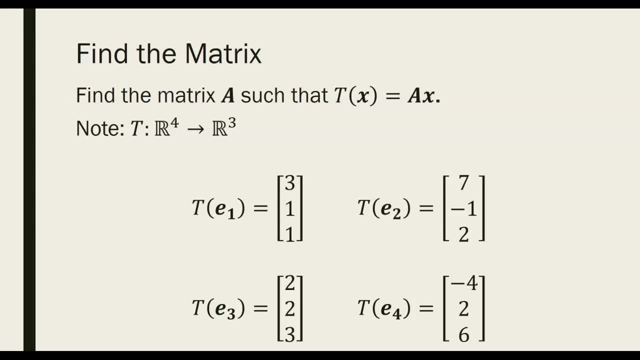 All right, In this case, We're going to go from R4. To R3.. All right, So We're going to go from R4. To R3.. All right, So We're going to go from R4.. 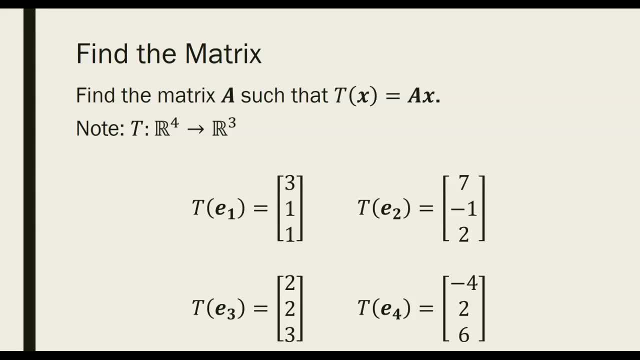 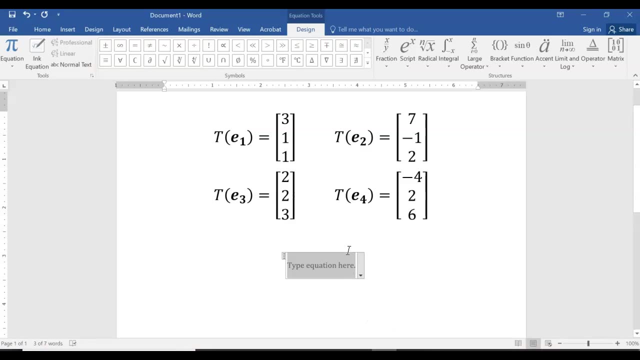 To R3.. All right, All right, So We're going to go from R4. To R3.. All right, Hopefully You did that. All right, So Hopefully You Went ahead And did that And got it. 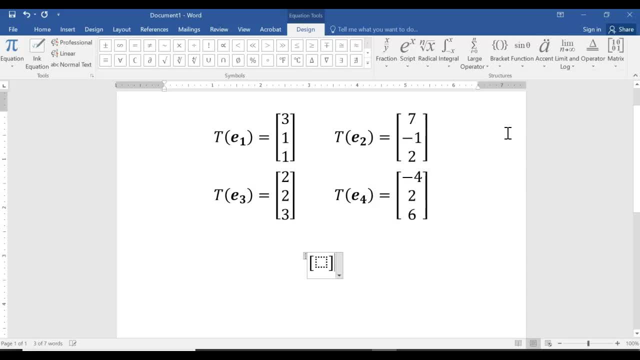 Now Let me just go through it In a fairly Quick way. When We're creating this matrix. I'm not going to go all through the Things, But Basically We're going to have an E1.. An E2.. 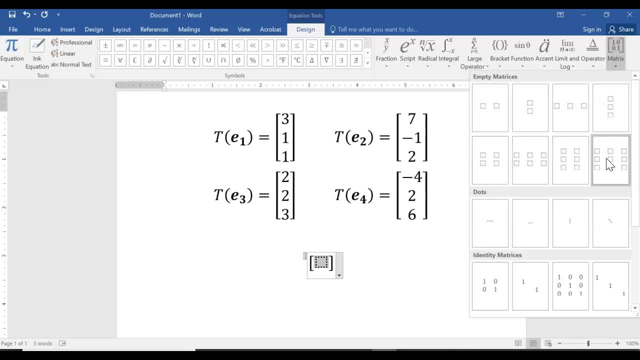 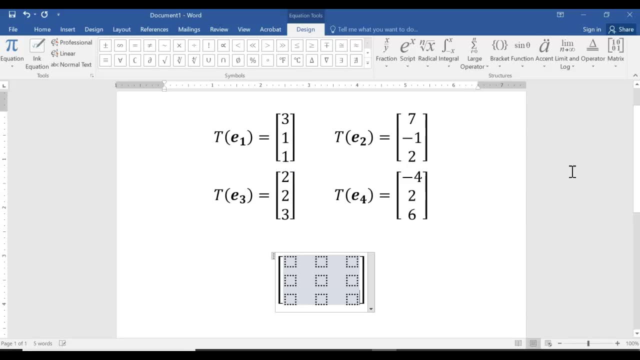 An E3. And an E4. That means We're going to have Columns And, Since Our outputs Are all In R3. That means We're going to have Three rows. Okay, So My matrix. 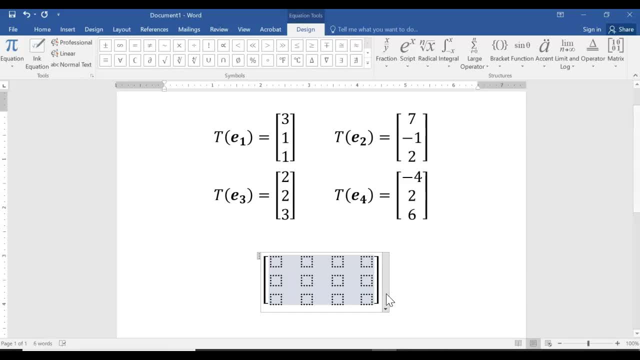 Is going to have Four columns And three rows. It's going to be a Three by four matrix And E1. Is going to My Image Of E1.. Is going to Determine My First. 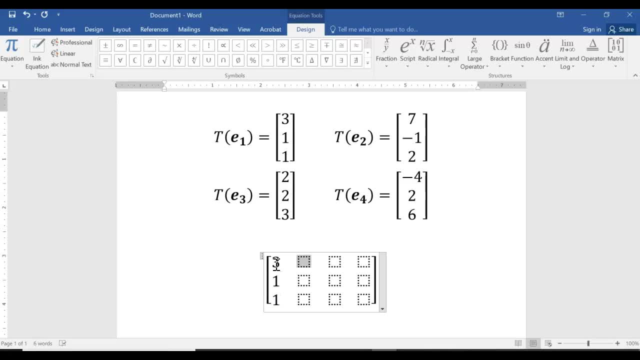 Column And My Image Of E2. Is going to Determine My Second Column. My Image Of E3. Is going to Determine My Third Column And My Image. 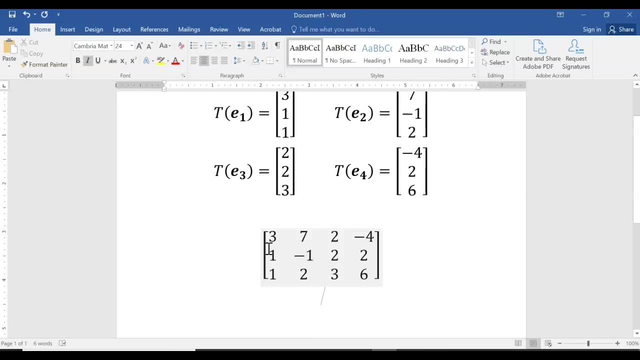 Of E4. Is going To Determine My Fourth Column. Okay, One, Two, Three, Six, All Right, So That's The Matrix That We Were Looking For. 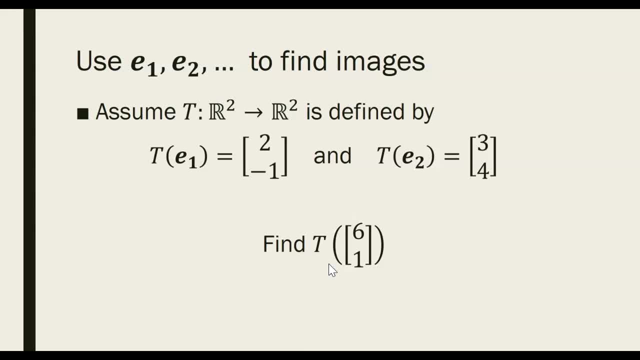 All Right, So The Other Thing We Can Do With This Fact Of The Transformation Is Linear: To Find Images Of Other Vectors. Okay, Now 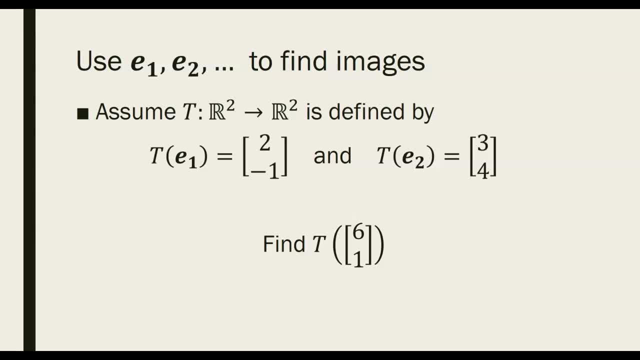 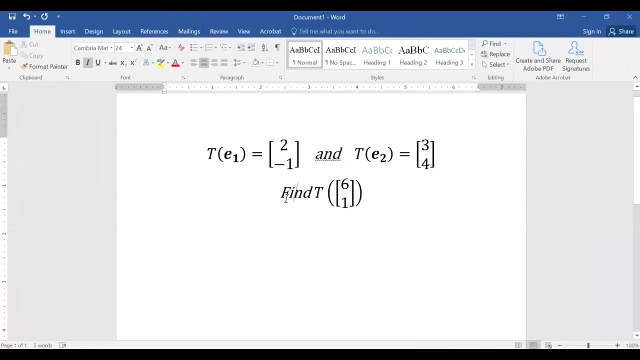 There's A Couple Of Different Ways You Can Go About This. I Will Kind Of Your Document Here And We're Going To Find T Of. 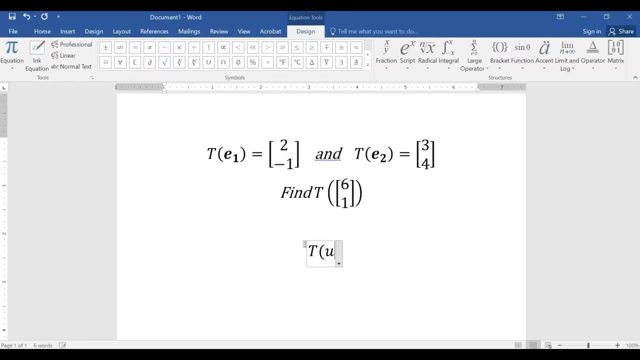 Six One. Okay, Now The Key, The Key Things We're Using Here, Is That If I Take A T- And Then Also We Know That- 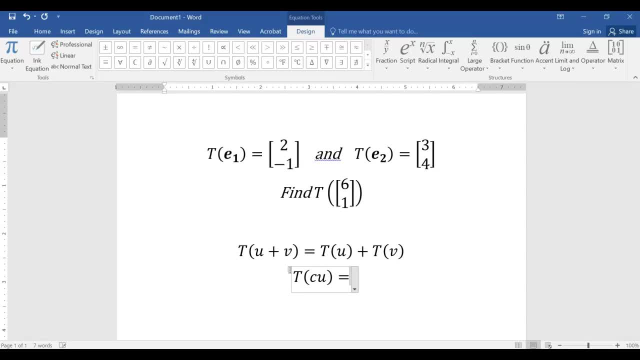 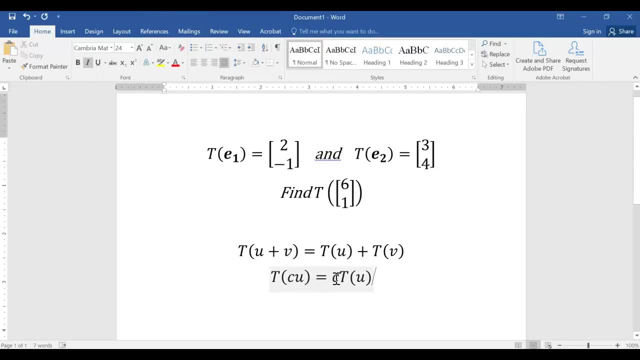 T Of C? U Is Equal To C? Of T? U, Where U? And V Is A Vectors And C Is A Constant. Okay, So 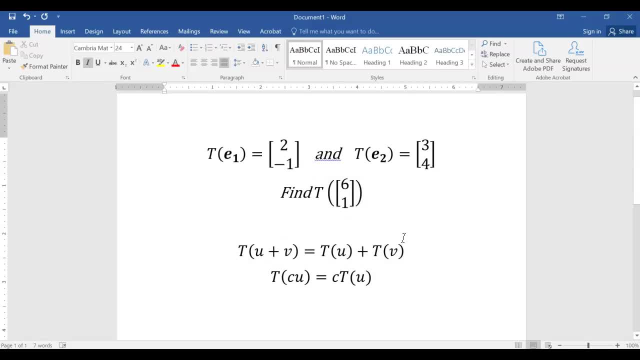 This Is The Image Of Six. One Is All Right. So This Is Sort Of Technique. One Use The Properties Of Linear Transformations That We 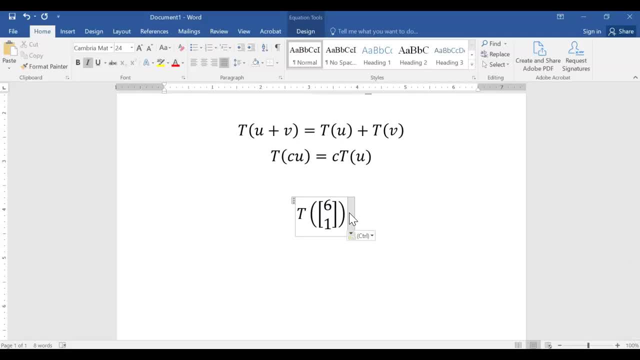 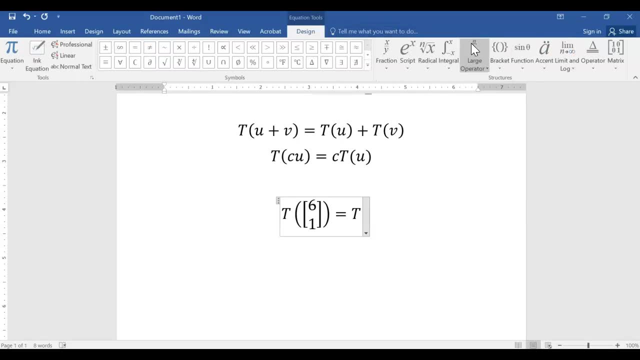 Know To Find Of Two Vectors, Specifically Vectors E One, And Just To Remind You Of What E One Was. E One Since We 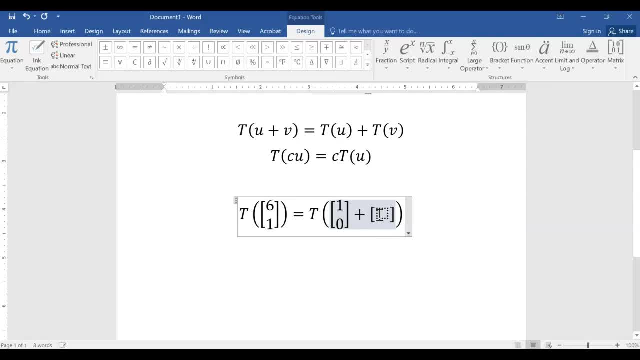 Are In E Two, So We Want To Write Six One As A Linear Combination Of One Zero And Zero One. Now That's Pretty Easy. 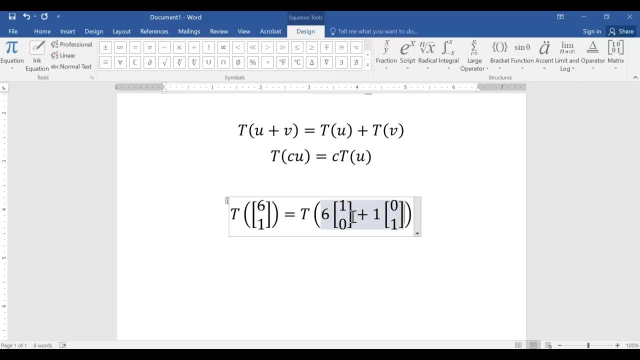 To Do. You Can Call That One Zero, You Can Call That E Two. It Doesn't Matter Which Way You Do That. If You Would, 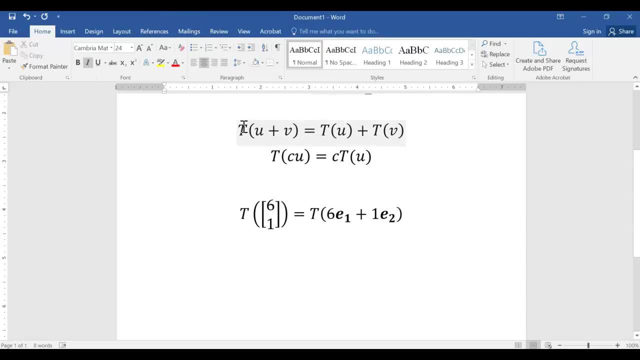 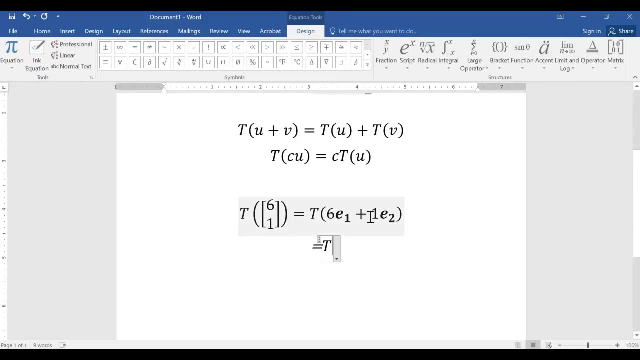 Rather Use The Terminology E One. What I Can Do Is I Can Break That Up And I Can Say: Well, That's Actually Equal To 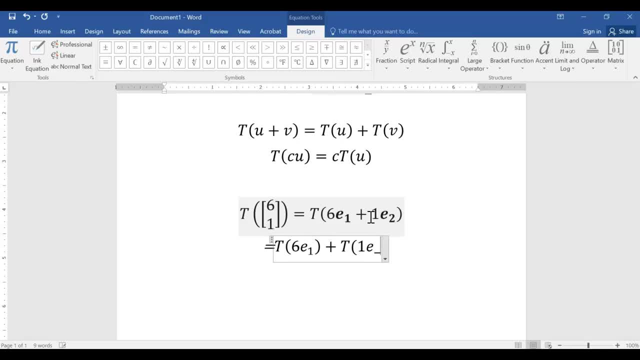 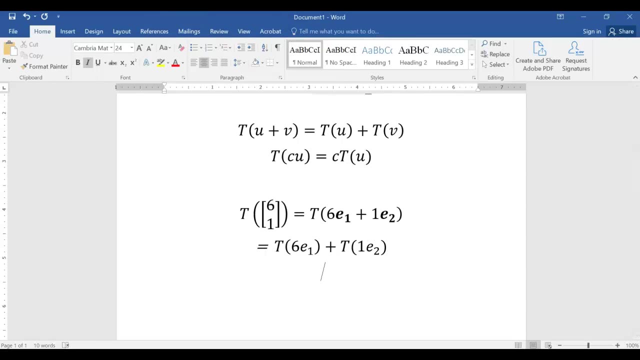 T Of Six Times E One Plus T Of One Times. You Can Break This Over The Sum. The Second Property Says: Well, You Can Pull. 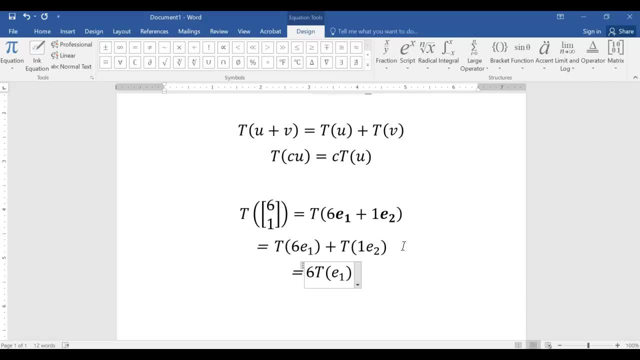 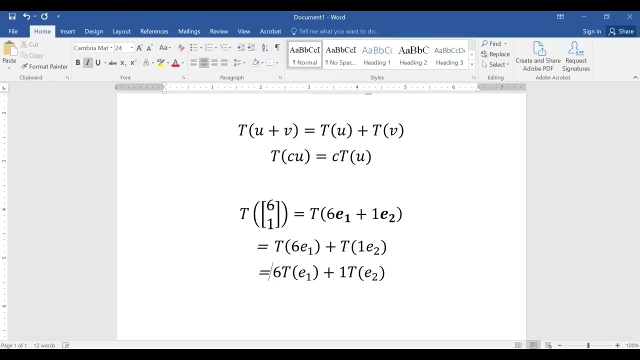 Out The Scalers, And So It Is Six Times T Of E One I Know Now We Know What T Does To E One Gives. 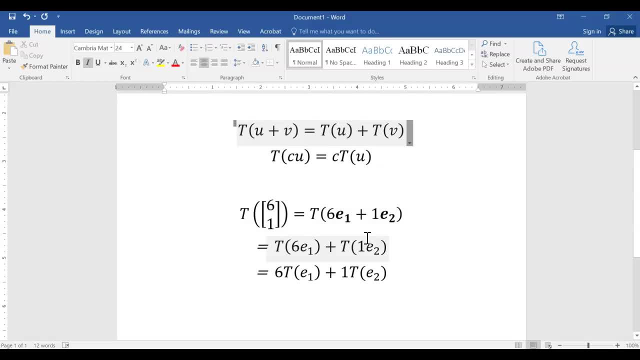 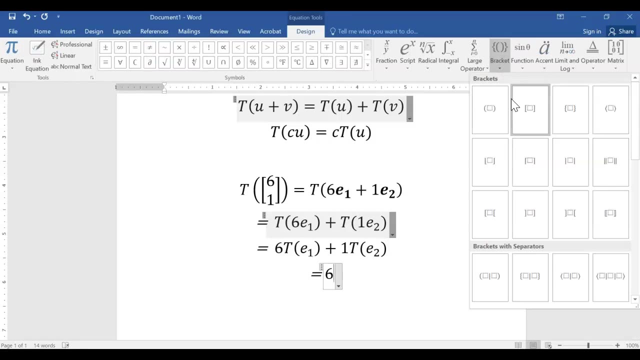 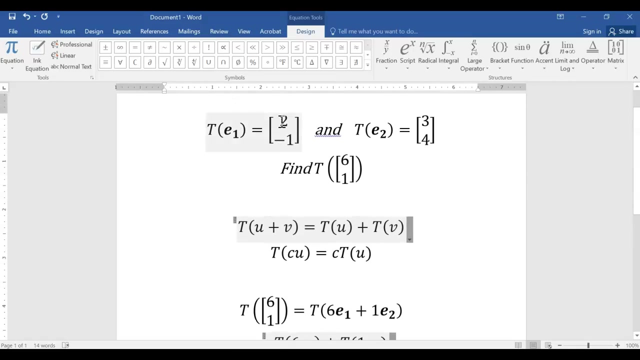 Me Two Negative One. We Know What T Does To E One Gives Me Two Negative One. We Know Times The Vector. Again Two Negative One. 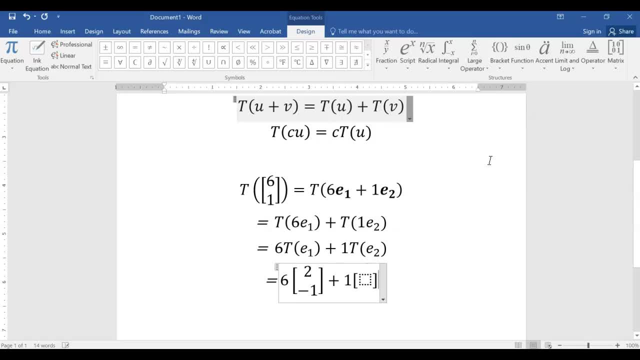 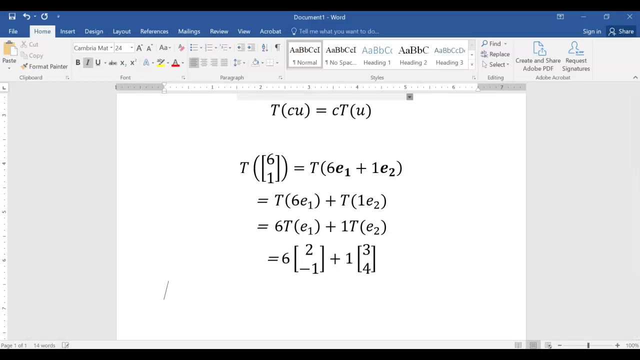 Plus One Times The Vector Three, Four Again. I'm Getting That Because Three With T, With The Transformation T, And Now It's Just A Matter. 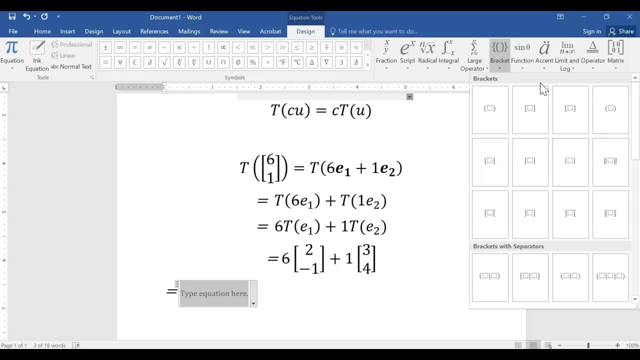 Of Computing With Using Vector Addition And Scalar Multiplication. So Our Resulting Vector Is Going To Be What? And Negative Six Plus Four Gives Me. 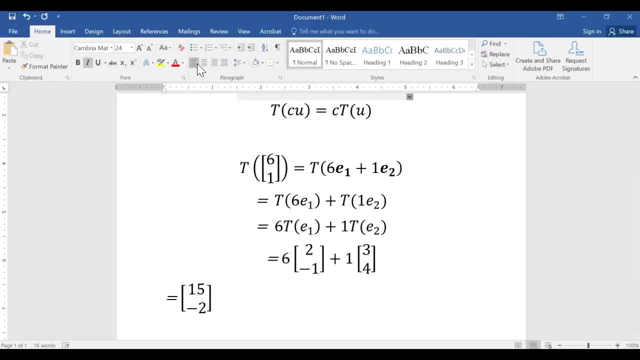 Negative Two. So, Without Even Having To Go Through Figuring Out Lots Of Things, Basically If You Know What A Transformation Does To Any Vector. 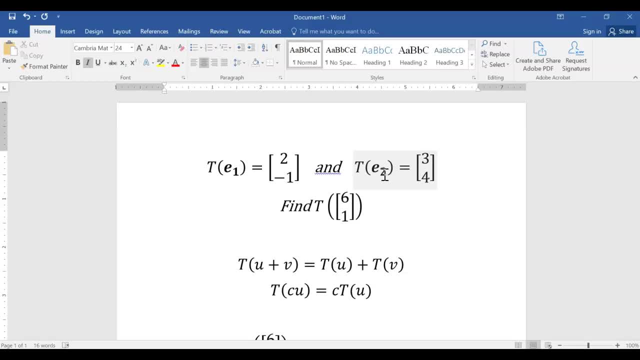 Because You Can Write Any Vector As A Linear Combination Of E1., E2.. E3.. Okay, Remember, E1. Is Just Basically Giving You A First. 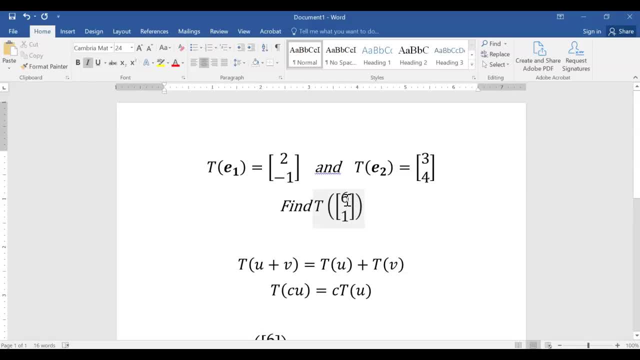 Entry Of One, Because The First Entry Is Gonna Be Again. First Entry Here Is Six. So When I Write A Linear Combination, It's Gonna 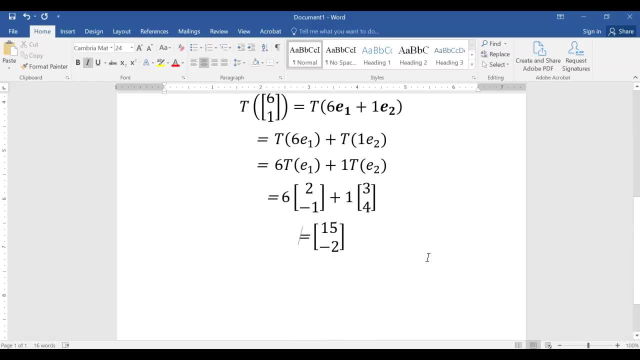 Be Six Times E1.. Second Entry Is Just A Linear Combination Of E2. And A Linear Combination Is Just One Entry Of E1. So 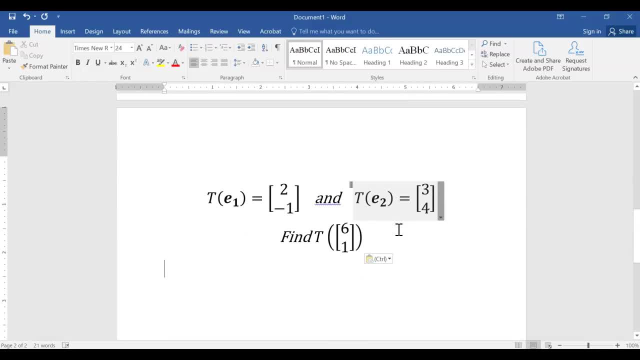 Let's Find The Matrix And Then Let's Compute T Of Six One By One. It Goes Like This: Start By Noticing That The Matrix 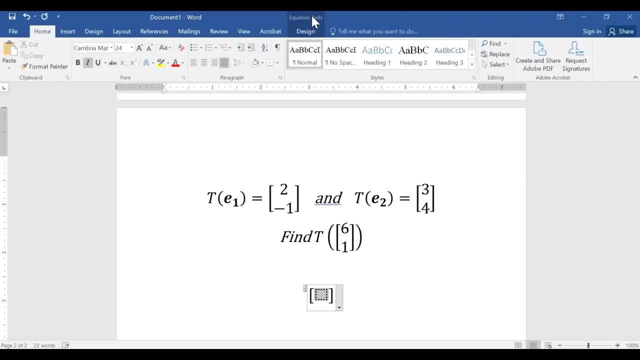 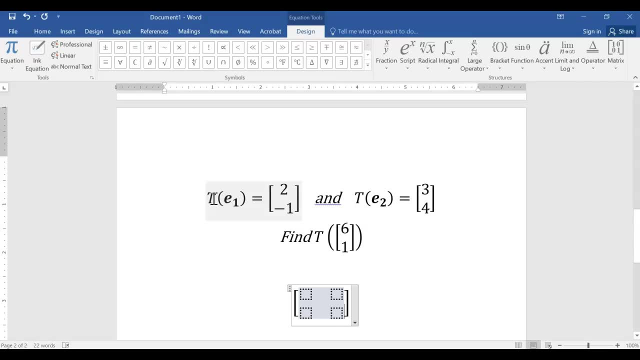 That I'm Gonna Get. It's Gonna Go From R2. To R2.. So It's Gonna Be Two By Two Column When I Multiply. 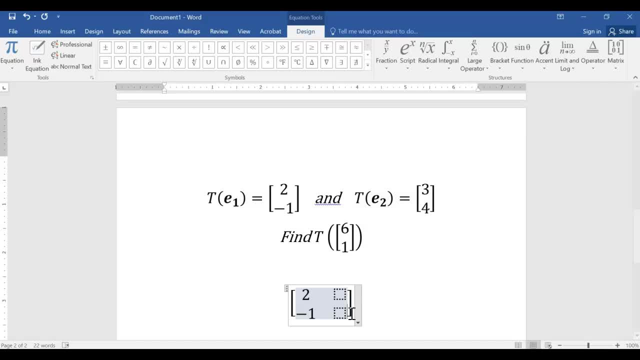 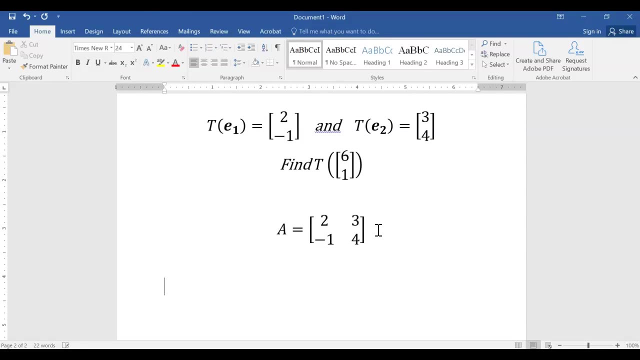 The Matrix Times, E2.. I'm Gonna Get The Same Thing As Taking The Transformation Of E2.. So That's Gonna Pull Off My Second. 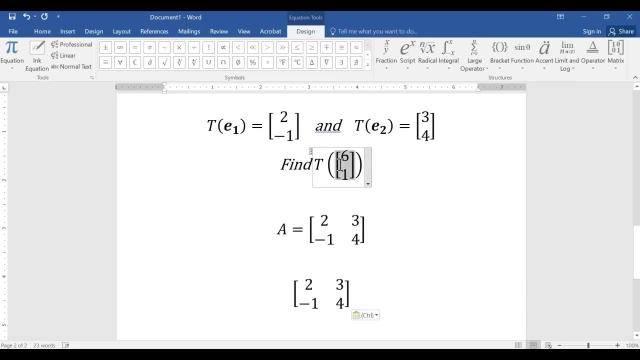 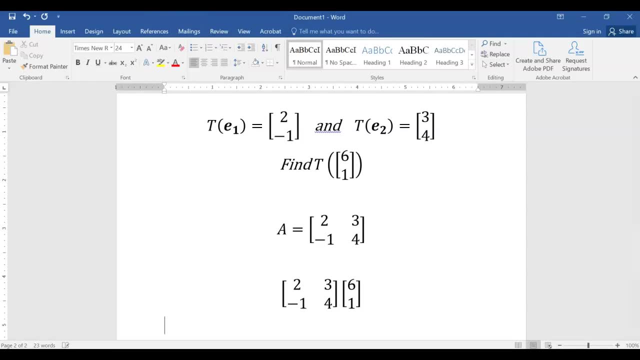 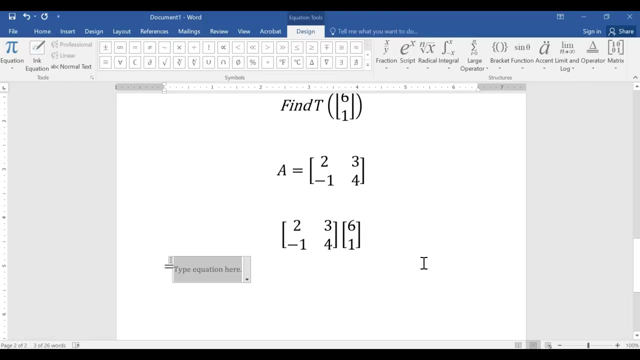 I Can Take A And I Can Multiply It, Times The Vector Six One And Get Out Some Answer Whoops. So When You Take A, 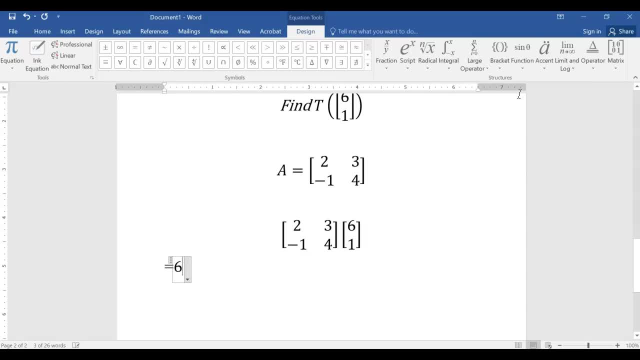 Times Six. One, I Guess, Times The Vector. Two Negative One. My Apologies, I'm Right In Bed Today. So Two Negative One Times Six Plus. 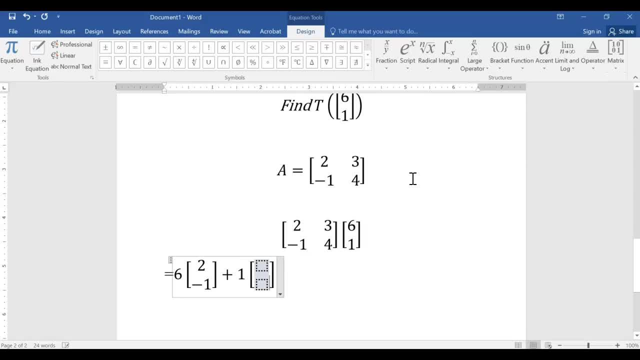 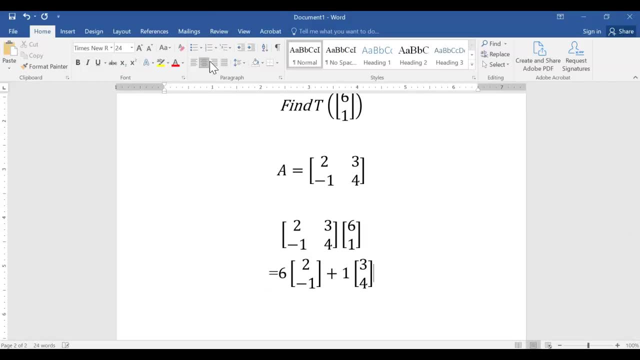 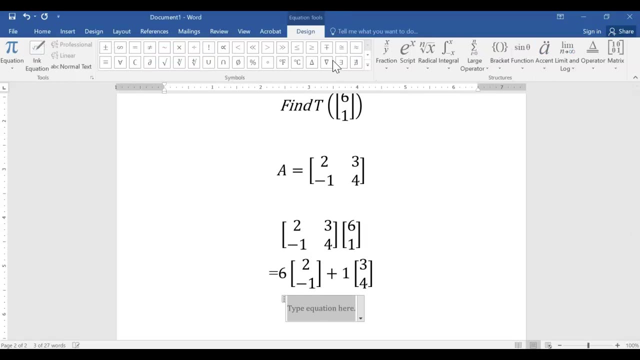 One Multiplied Times The Vector And Again It's Fairly Obvious That We Are Getting The Exact Same Result. In Either Case We're Getting. 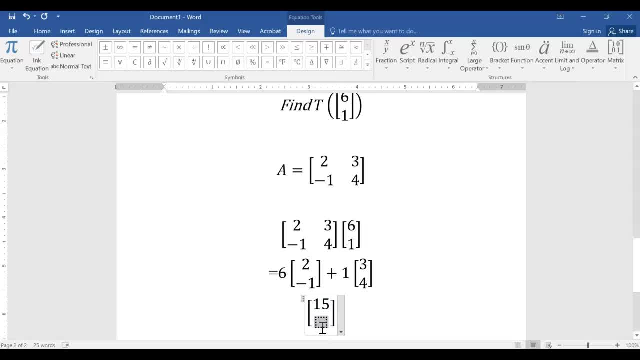 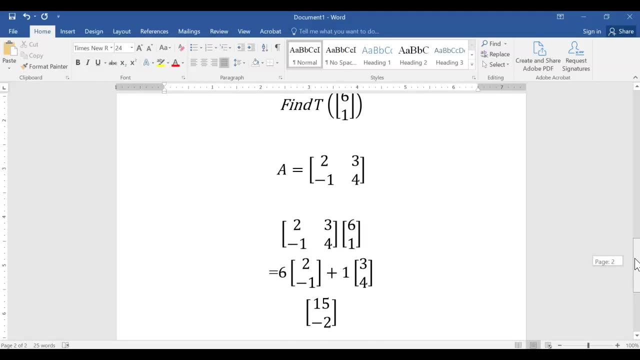 The Vector Which Has A Fifteen In The First Entry Is Fine With Me If You'd Rather Use The Method Of Utilizing Properties Of. 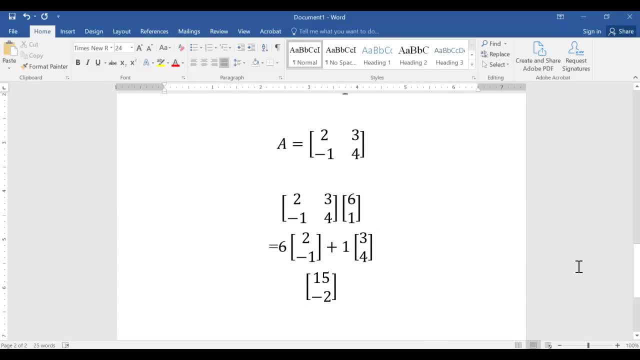 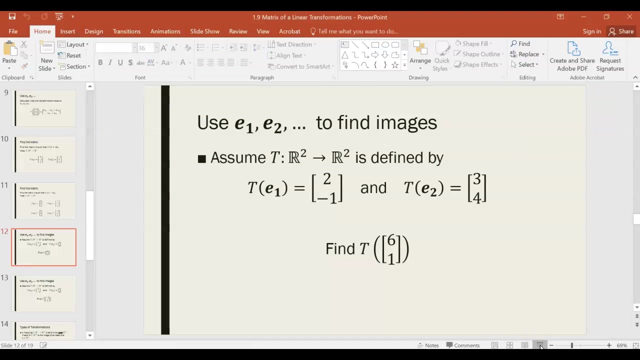 Linear Transformations. You Can Break Down That Way If You Would Rather Utilize Finding The Both Methods, Ended Up With That Line There, Okay So. 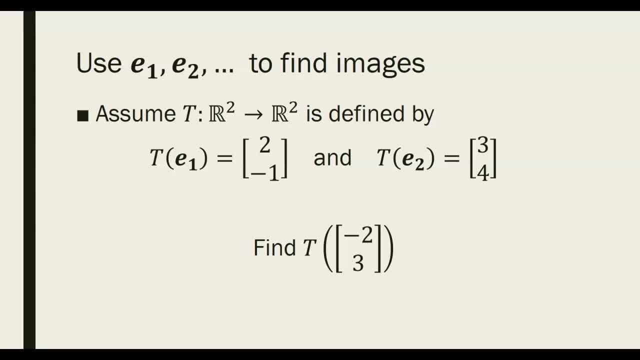 That's The Important Thing. So What I'd Like You To Do Is We're Going To Use The Same Transformation. All Right, It's Going To. 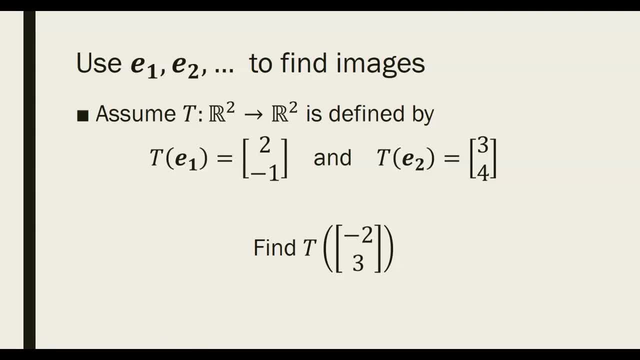 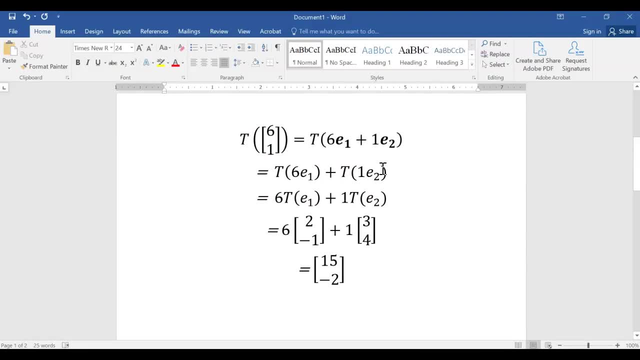 Look Very, Very Similar. Oops, Except Now We're Going To Use Negative Two, Three. So If Your Transformation Starts, Applies Hits Negative Two, Three, All. 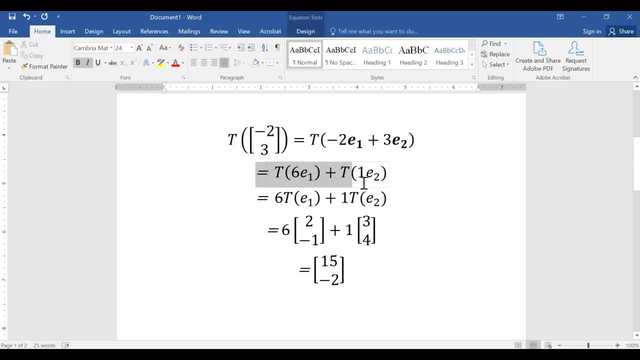 I Have To Know Is That My I'm Going To Skip This Step. So All I Have To Know Is That I'm I Can Break. 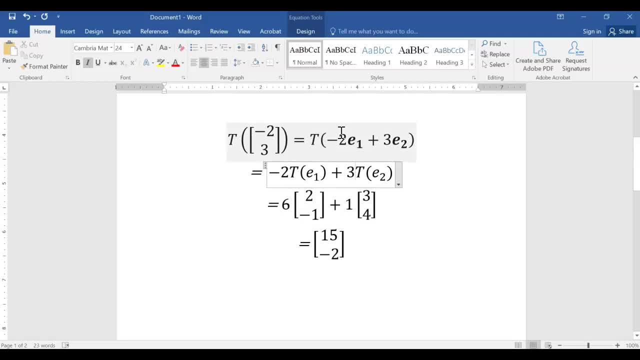 The Transformation Up Since Applied To E2.. Times Three Is Going To Give Me My Result And We Just Use Different Numbers Than We Had. 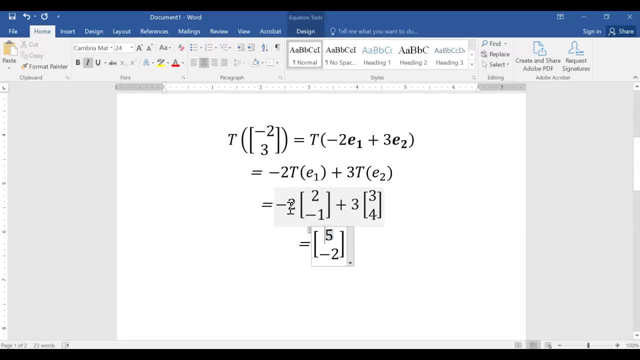 Last Time. But The Same Concept, Negative Two, Three Times Four. So Two Plus Twelve Gives Me Fourteen Right, So You Could Have Done It. 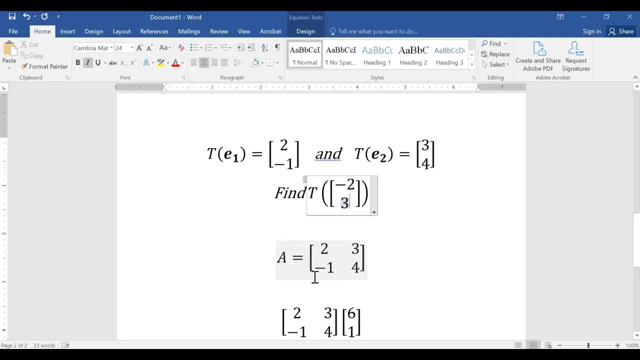 That Way You Could Have Also Done The Matrix Way, And So You Get. In Either Case, We're Getting The Exact Same Thing We're Getting. 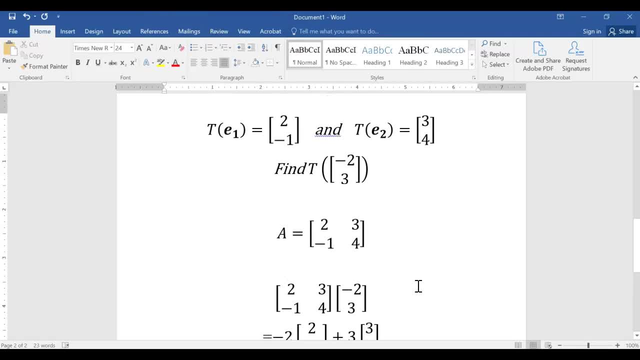 Them That When You Take Negative Two, Three, Hit It With The Transformation You're Going Of Negative Two, Three. Under Transformation, T Is Five Fourteen. 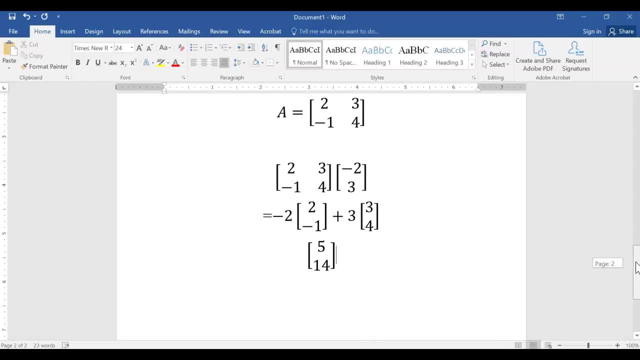 So Though That's Sort Of A Nice Way To Use Those Ease, Okay, Again, These Are What Are Going To That, What We Call E. 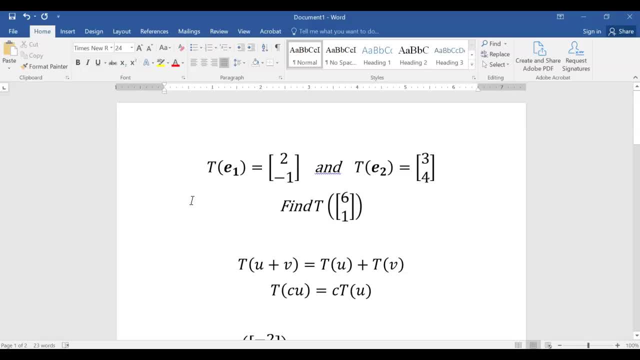 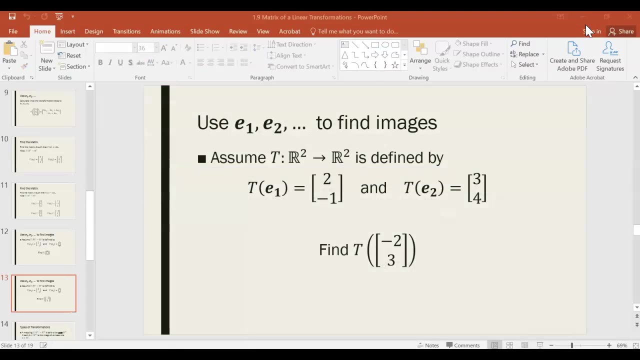 Sub One E Sub Two In This Class Will Always Be Those Vectors, A One Or A One In Entry One And Zeros Elsewhere. 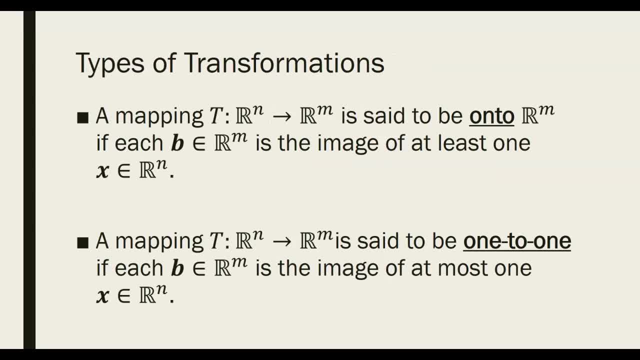 Of Negative Two, Three Under That Transformation. Now One Thing We Want To Get Into Is We Want To Look At Some Different Types Of Transformations. 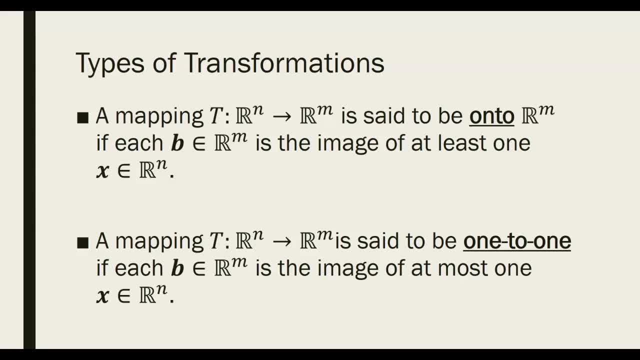 Specifically, We Want To. So Let's Start With The Idea Of On To We're Going To Have A Transformation That Goes From R N To. 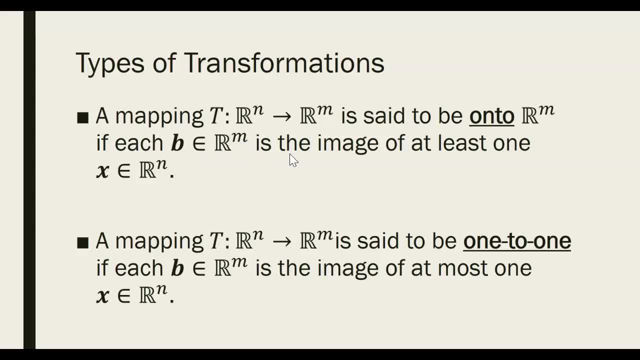 R M. So R M Is My Codomain, All Right. Another Way To Say On To Is That The Range Is Your Codomain, Okay So. 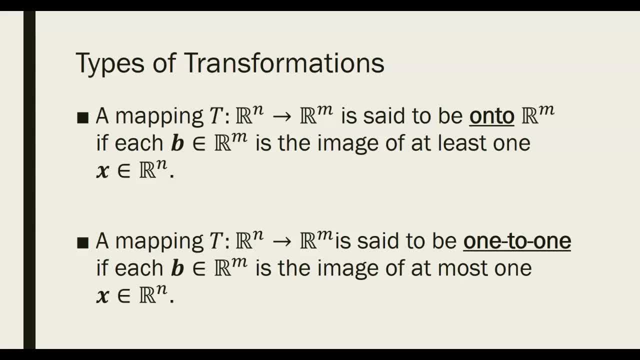 Every Vector In R M Can Be Formed As A As An Image In My Codomain. Now A Mapping Or Transformation Is One To One. 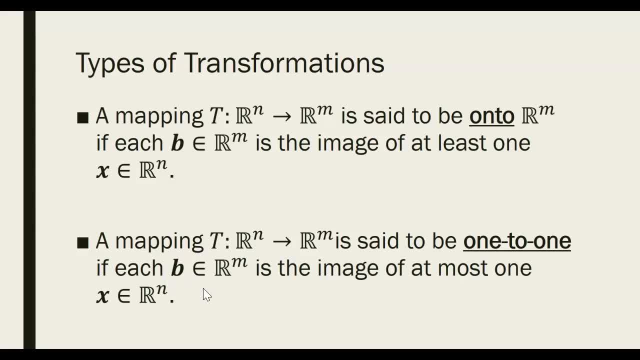 If, When You Find A Vector In Your Range, Or Let's Say For Every Vector In Your Domain, Okay, So This Is At Least One. 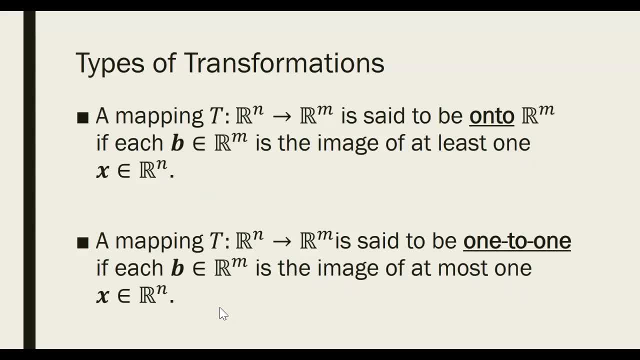 Vector. This Is At Most One Vector. Okay, So Here's The One To One. What One To One Basically Means Is So One To One. 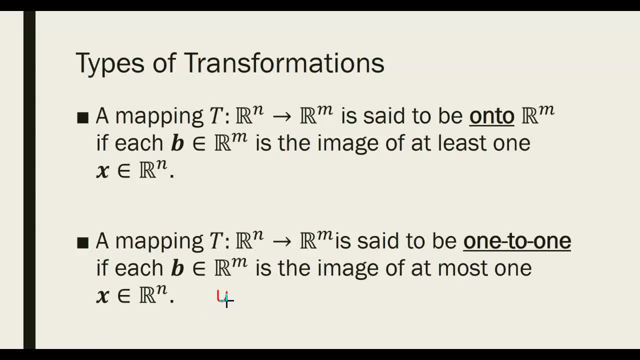 Means That If You Were Drawing This, If You Had For Instance A U And A V In Your Domain And They Both Mapped To. 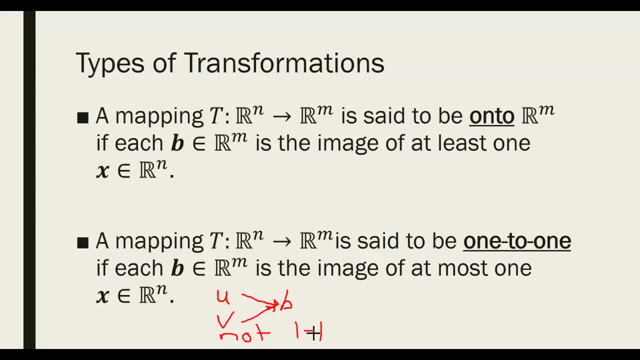 Your One, Sometimes One To One. We Shorthand Is One Dash One, Or One T O One. Okay, So What We're Going To Do Is 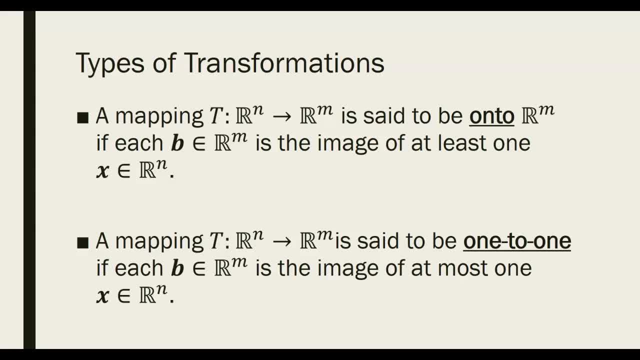 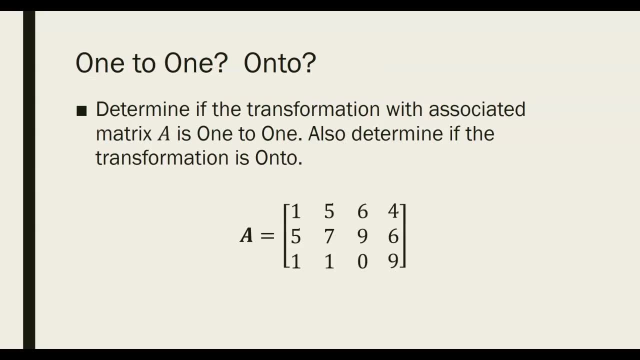 We're Going To Look At A Vector In My Domain, Okay, So Let's Take This Matrix For Example A. You Can See The Matrix There. 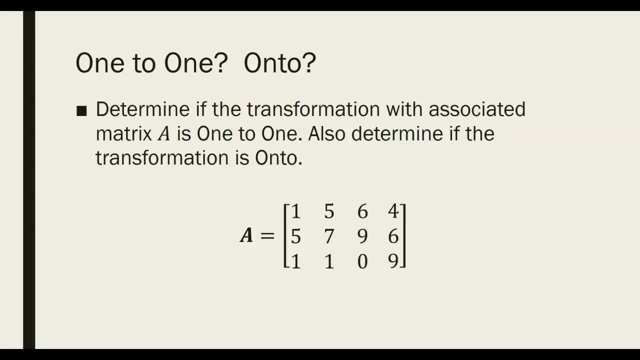 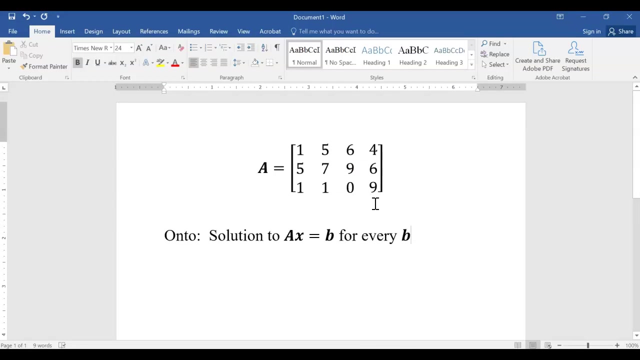 We're Going To See If Now The Way To Do This Is To Use Techniques That We Saw Earlier. So The Technique That I'm Talking. 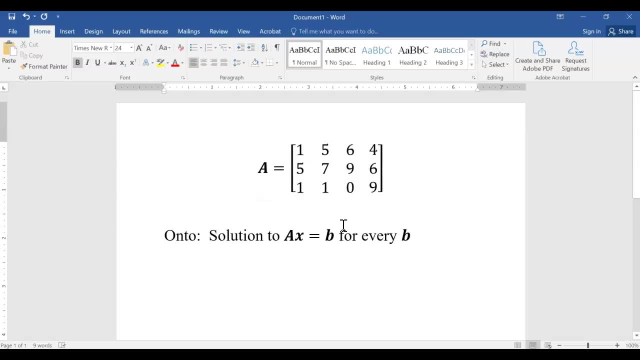 About That We Did. Earlier Is Thinking About Again. Think About What On To Means In Terms Of A Matrix Equation. So We Have This Matrix. 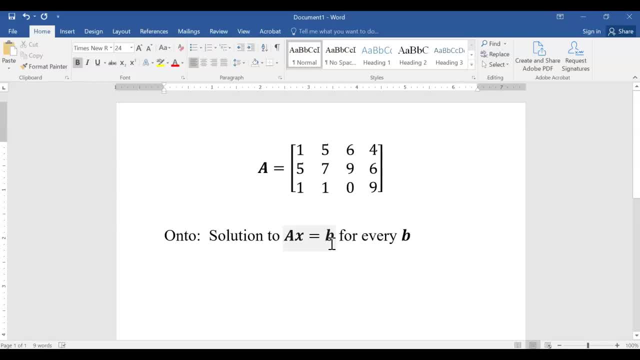 Here A Now On To Means That For Every B That You Can Think Earlier And All We Have To Do Is Put A Into Row. 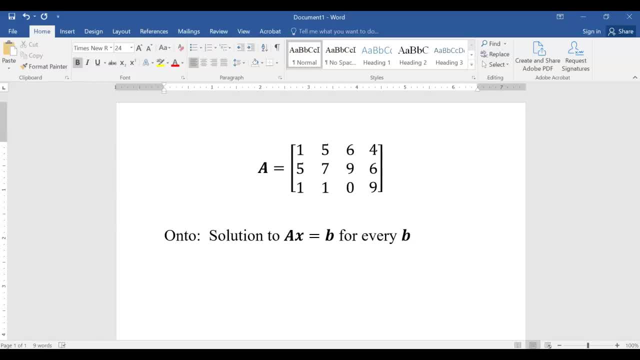 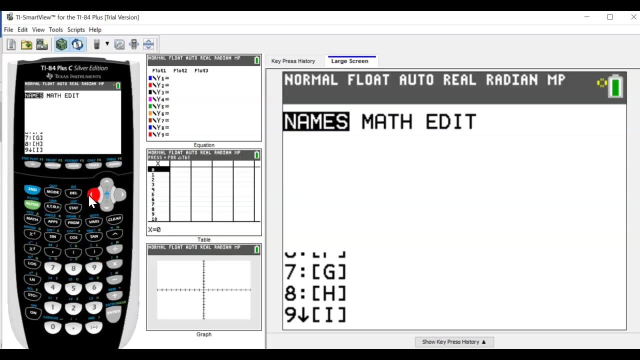 Reduced Echelon Form And Then Think Through What Kind Of Solutions We Could Get, What Kind Of You Plugged In A Matrix. So We're 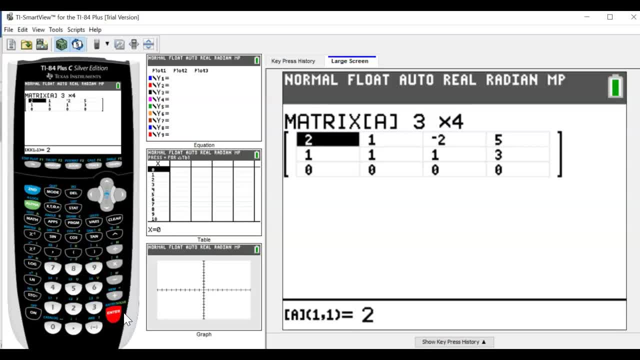 Going To Take A Matrix. Our Matrix Is Three By Four And Our Entries Were One, Five, Six, Four, Five Seven, Nine Six. One, One, Two. 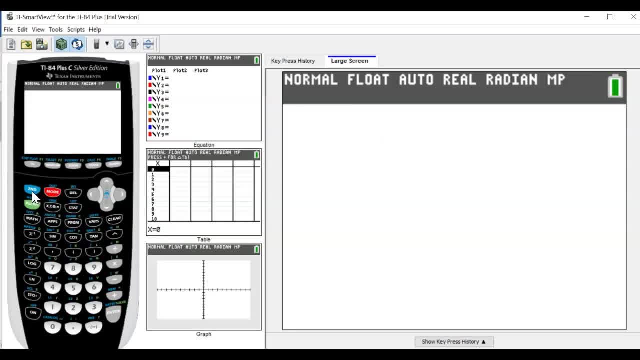 Three, Four, Five, Six We- We Think That We Did So Quit- Go Into The Matrix Menu One More Time. Math Row Reduced Echelon Form. 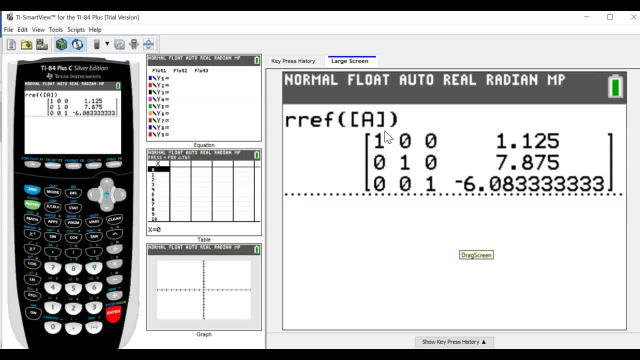 We're Going To equation ax equals b for all b's. So what I would have done is I've left off the column over here to the right of all the constants, but no matter what this column over here to the right would have been. I'm saying like if we had an augmented matrix we would have had to add: 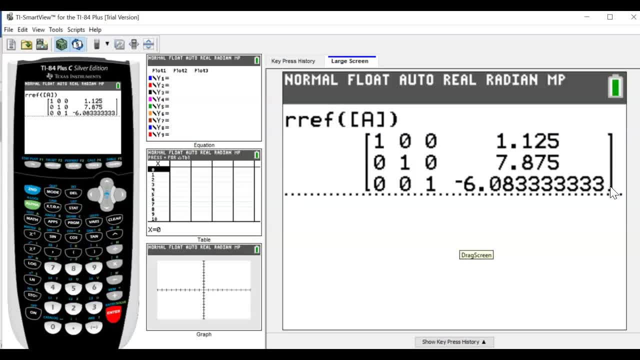 another column. So, whatever that column would have been, we could have found answers. all right, no matter what that would be, because each row has a pivot position, So we could have found answers. In fact, we could have found infinitely many answers. 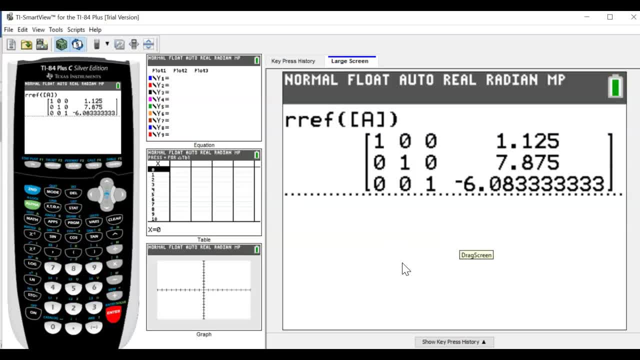 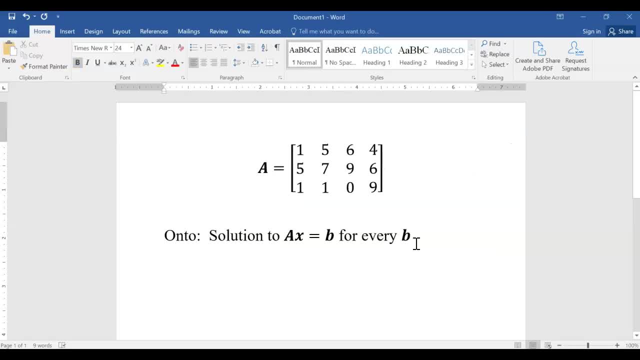 for pretty much each b that we choose. all right, So in the In this case, since we can find a solution, we can- whoops, can- find a solution for every b. we know the transformation is onto. Okay, so that's it. 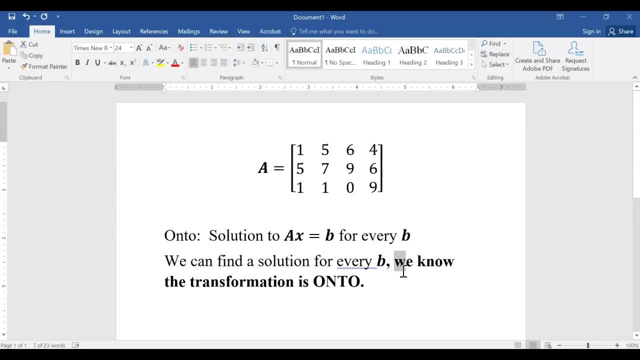 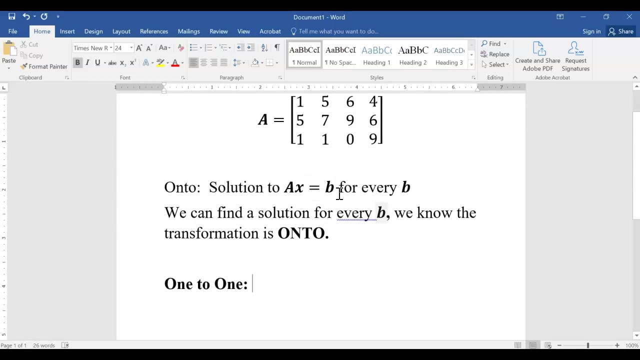 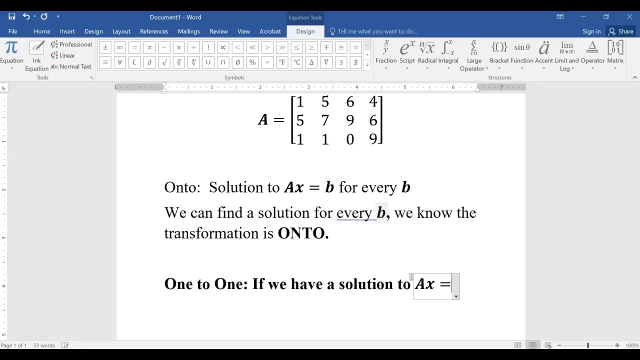 Let me unbold that. And there we go. Okay, so this is onto Now. think about what one-to-one means. All right means that if we have a solution, there is only one. If we have a solution to the equation ax equals b. 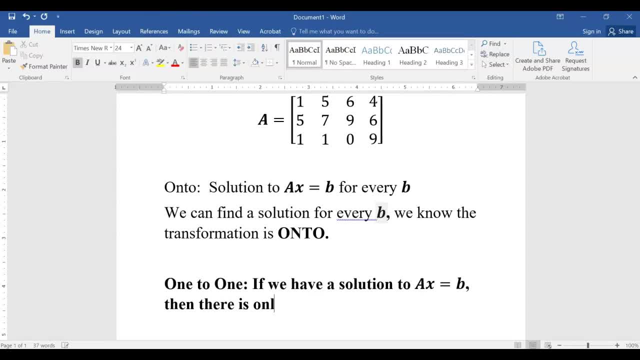 then there is only one such solution. Okay, So the key here: if there's one solution, then there can only be one. There can't be multiples. all right, Now what does the row-reduced form of our matrix indicate? 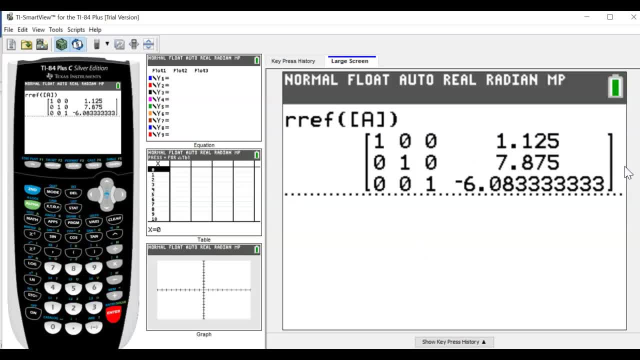 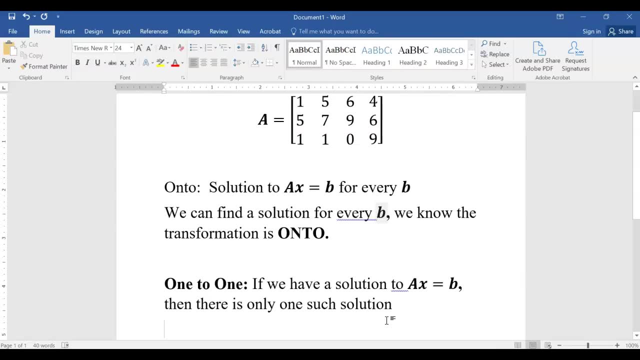 Well, it indicates that there's going to be an infinite number of solutions, no matter what these b's are. Okay, this column here represents a free variable which represents infinitely many solutions. So when we row-reduced, we can find infinitely many solutions for some b. 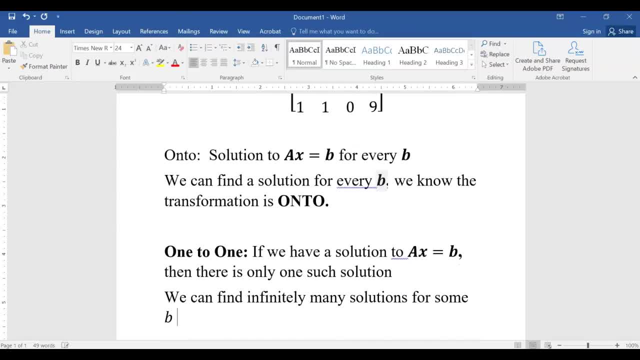 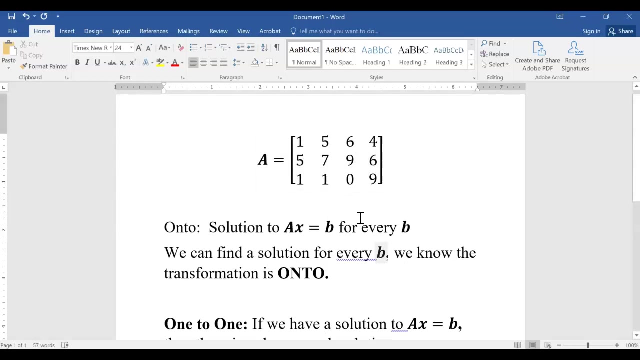 So the transformation is not one-to-one. Hopefully that makes sense. So infinitely many solutions, therefore, not Not one-to-one, okay. So this matrix transformation, this transformation that was represented by this matrix, I should say. 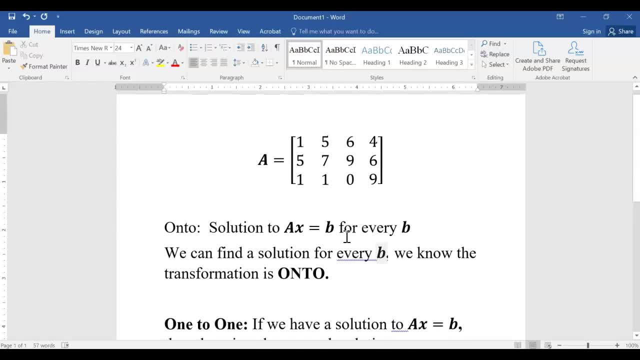 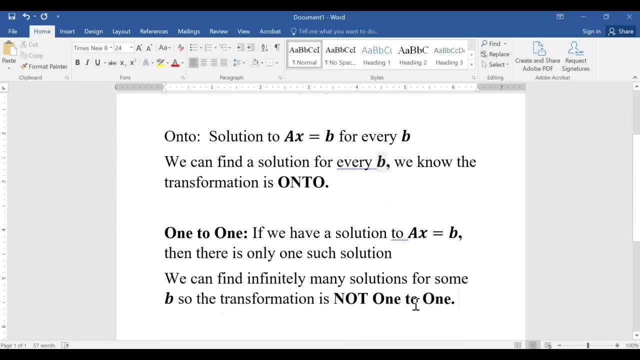 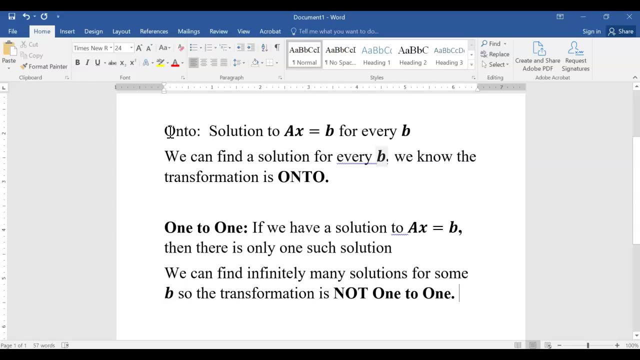 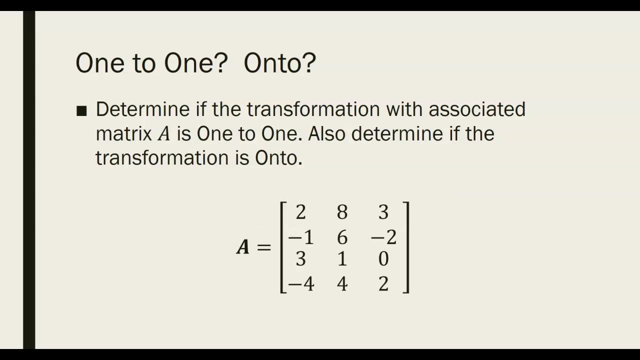 was onto because you could get every b but was not one-to-one because there were infinitely many ways to get to some b's. all right, I should not have bolded that. maybe I don't know. So I would like you to try think through this next problem on your own. push pause on the video. 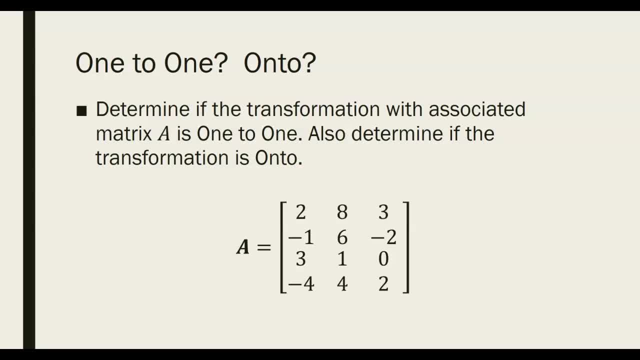 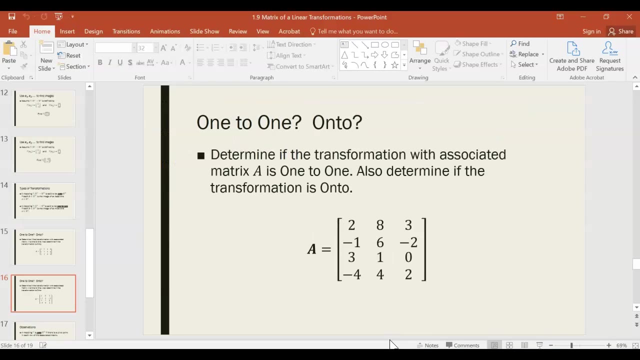 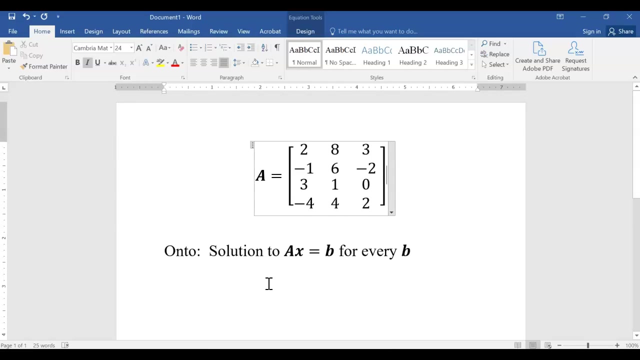 and see if this, the transformation with this associated matrix, is one-to-one and whether this transformation is onto. All right, hopefully you went ahead and did that, okay. So basically we'll do onto first. If you did one-to-one first, it's fine. 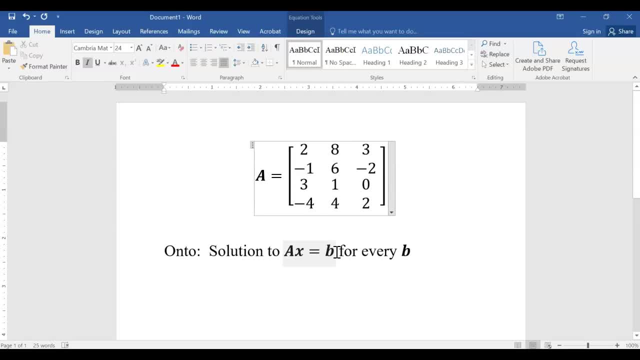 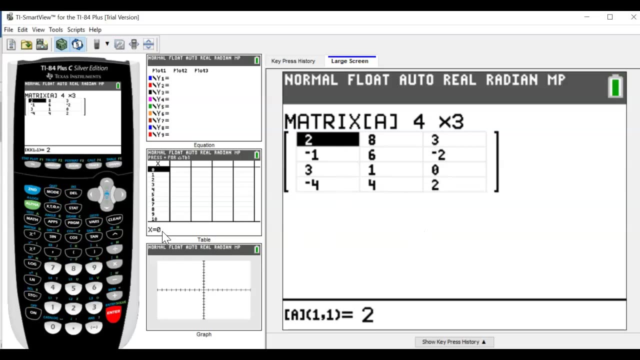 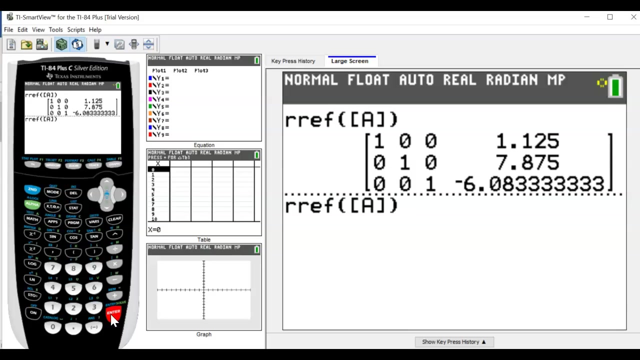 We're going to say: is there a solution to this matrix equation for every b that you can think of Again, think augmented matrix. We'll have another column here. Odd, I took the matrix A and threw it in my calculator. When you put it into row-reduced echelon form, watch this. 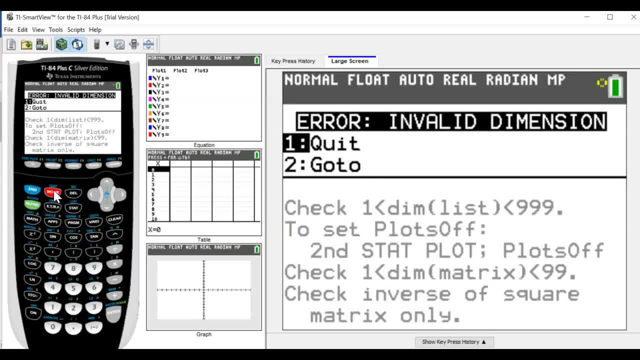 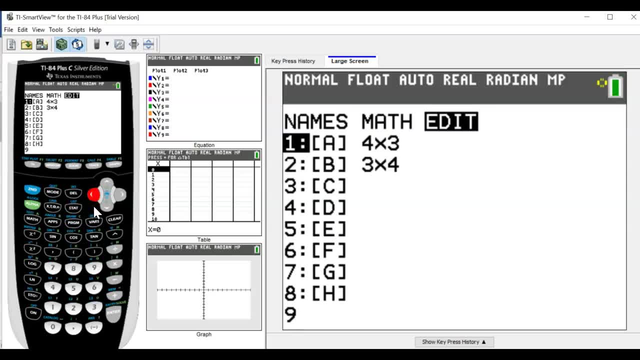 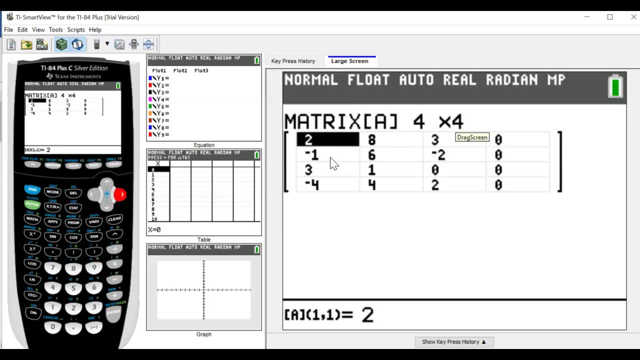 it's going to give you an invalid dimension. We've done that before, So what does that mean? That means we have to add in a dummy column. Hopefully you remember that, Because I have more columns than rows. our calculator for some reason doesn't like that. 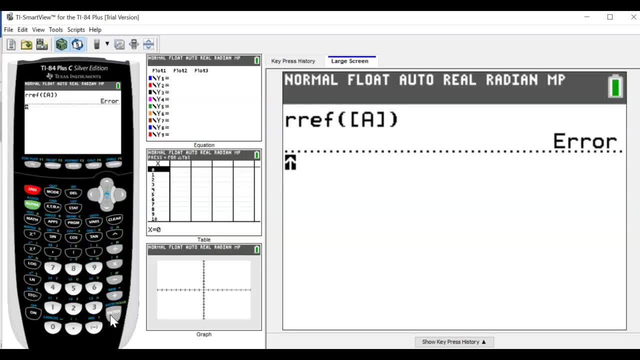 You can still sort of get around that fact by just throwing in that dummy column, But what you'll see is that, again, ignore this last column, you get ones on the diagonal. but you also have this row of zero, And if we had a last column here, we could put a one and get a no-solution case. 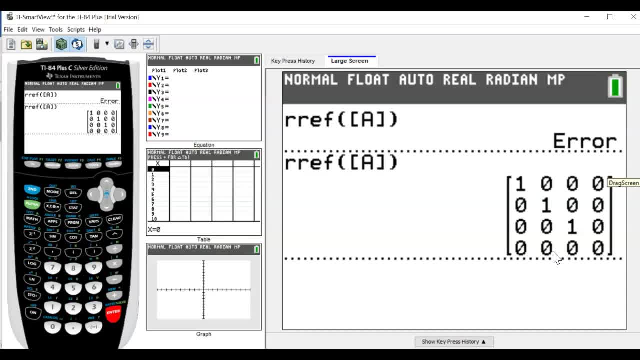 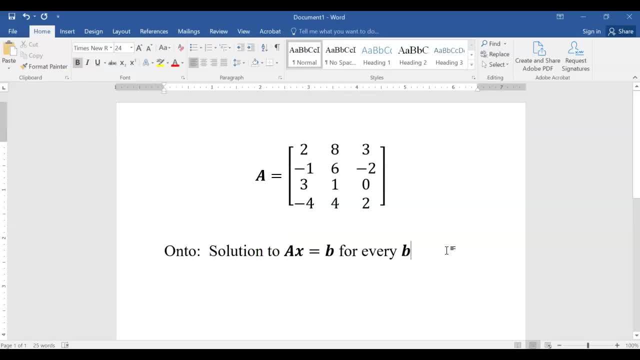 So there are cases here, because we could end up with zero on the last row equaling one. There are cases, there are situations where there would be a, b, such that it'd be a no-solution. So there are. 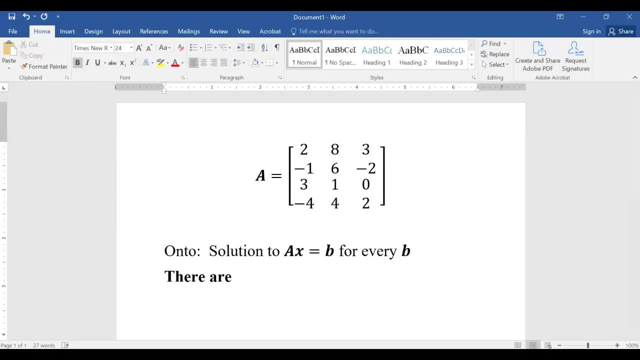 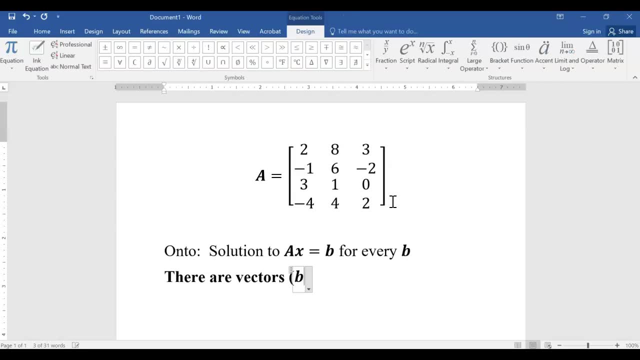 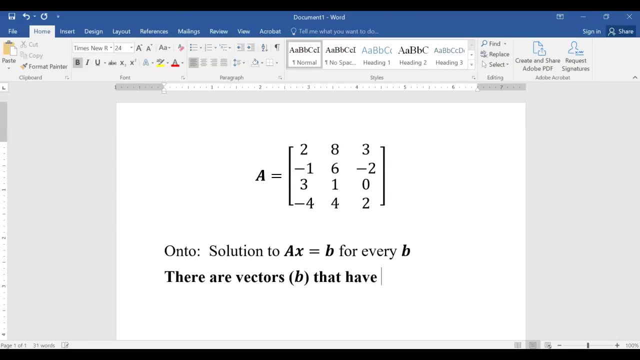 Whoops, Vectors, The b's specifically, That have no solution And therefore the transformation is not onto. So you can see that there's no solution. So you can see that if you have a solution, you're going to have a solution. 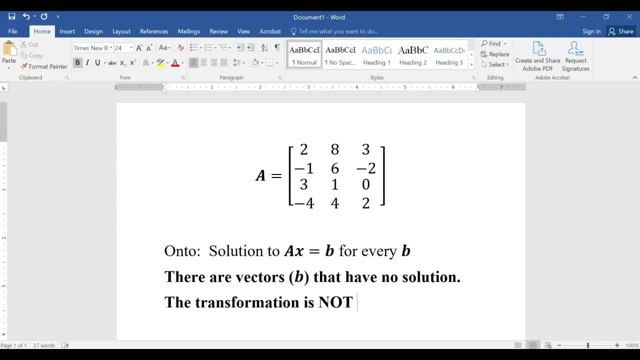 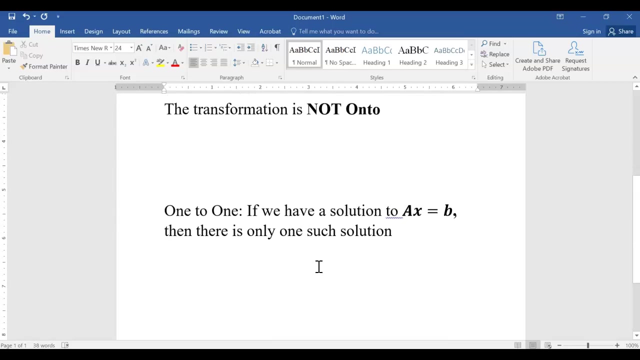 So if you have a solution, you're going to have a solution. We'll go capitalize that, not onto, So that's it. That's basically it. Now is it one-to-one? Okay, One-to-one says: if you have a solution, 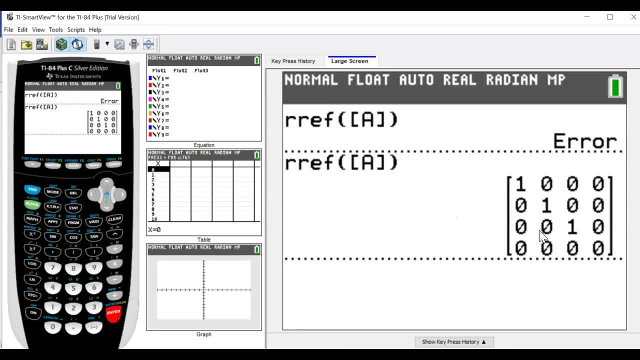 there's only one such solution. if you go back to this matrix again, this, this last column- don't throw think of that kind of pretend- we erase that last column. so we have three columns. each one has a pivot position. there are no free variables. no free variables means that every time there is a solution we only get one. 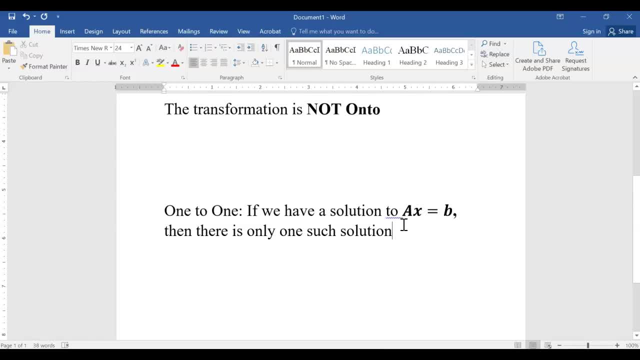 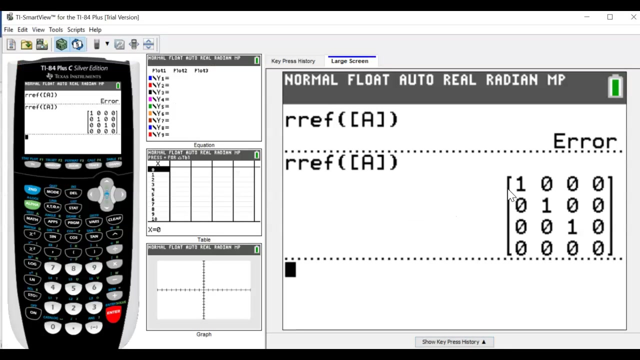 solution or we only get one answer. only get one answer when the equation ax equals B is solved, all right, and therefore the transformation is one to one, alright. so if there is an answer, there's no free variables, variables Again. forget that last column, That was the dummy column. 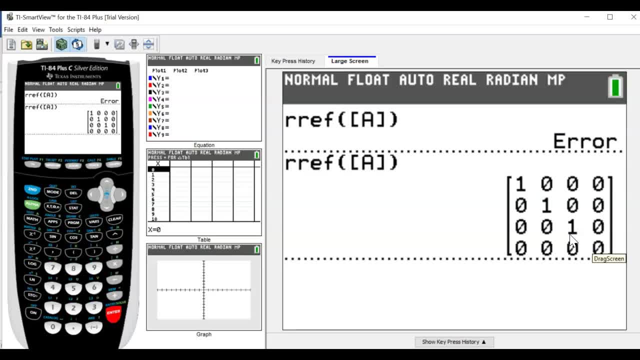 No free variables. so only one solution every time there is a solution. Now there's going to be vectors, that there's no solutions, We saw that. but that doesn't affect it. That does not affect one-to-one. Okay, one-to-one is not. 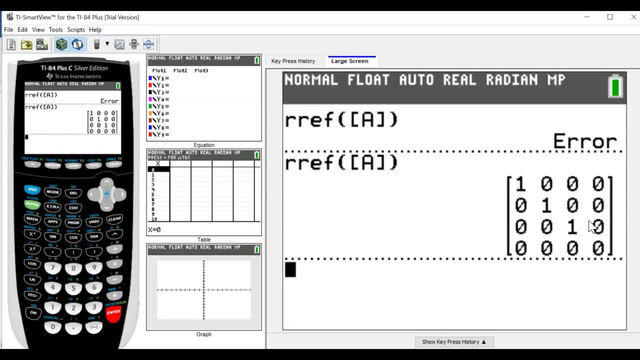 affected by which vectors you can get. It just says how many ways can you get them, And in this case, if there is a solution, there's only one of them. Now, just notice the types of matrices that we used. They were different sizes. 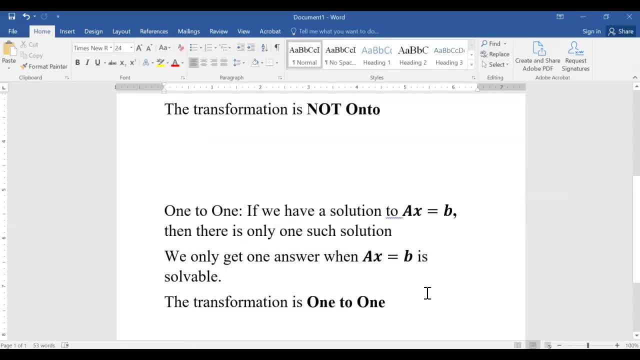 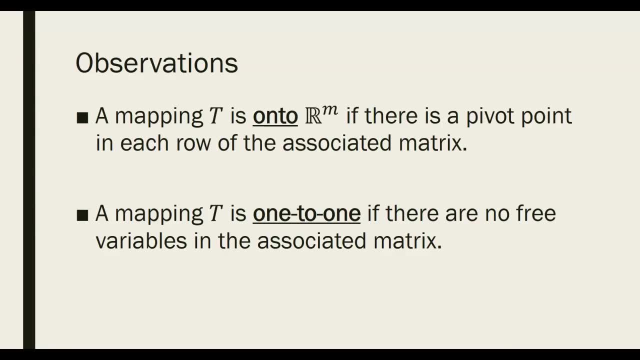 And they weren't square specifically, And that allows us to make some observations. Well, first off, let's make some observations about where the pivot positions were at. So a mapping is onto if, when you row, reduce it, there's a pivot point in every row. 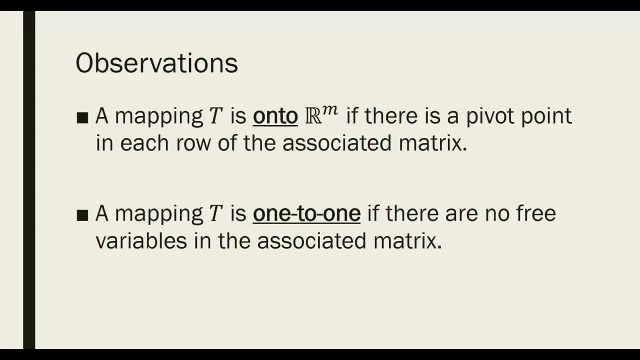 of the matrix. obviously, If there's a pivot point in every row, that means we can find a solution. If we can find a solution for every b, it's onto As far as one-to-one goes. well, one-to-one, it means there can't be. 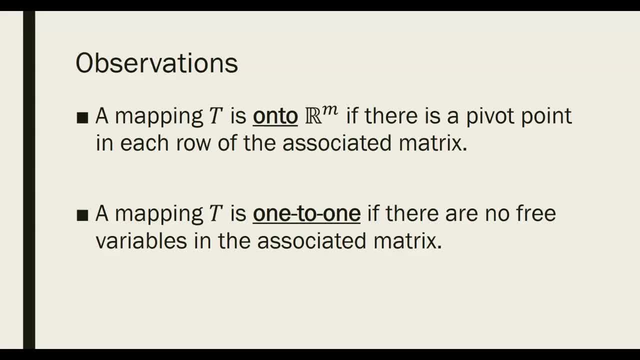 multiple ways of getting to the same vectors, And so if there's no multiple ways of getting to the same vectors, that means there's no free variables in our associated matrix. So hopefully that makes sense. Onto means there's a pivot point in each row. That's what we showed. 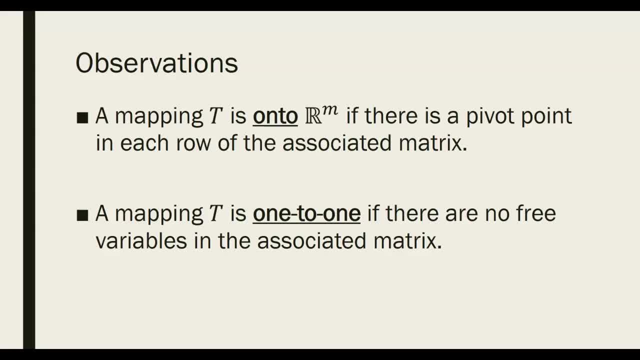 through that first example. The second example: that last row did not have a pivot point and therefore it was not onto As far as one-to-one goes. in the first case we had a free variable, so we were not one-to-one. 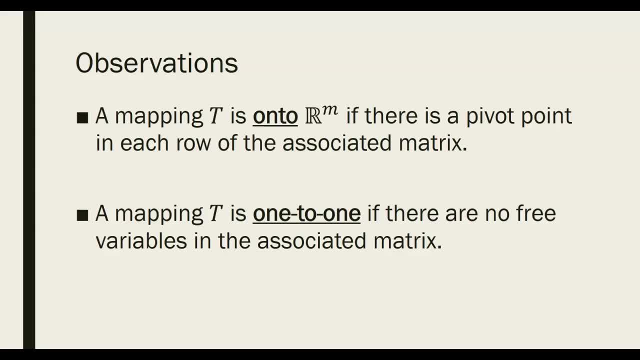 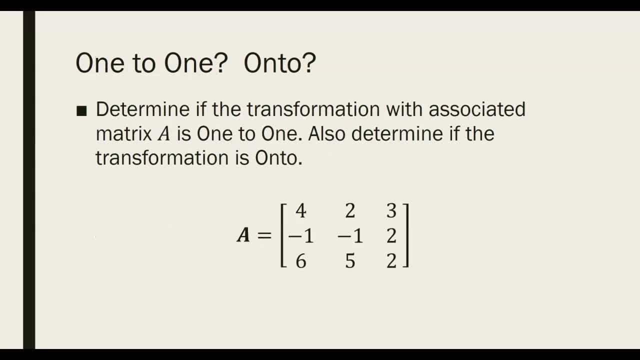 In our second case, there were no free variables, so it was one-to-one. So what I'd like you to do here is determine if this matrix is one-to-one and if this matrix is onto. Now, I just said it slightly wrong on purpose. 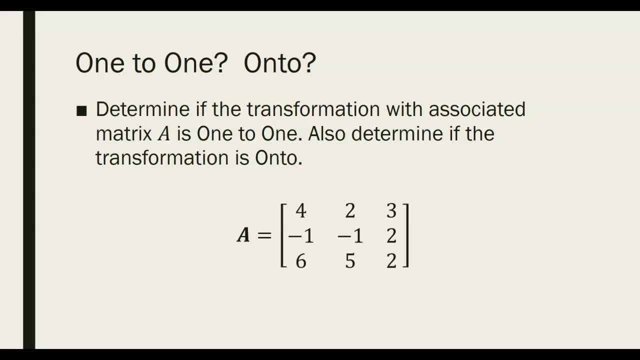 So technically the transformation is one-to-one and onto, but sometimes we will use sort of in this class, the bastardized language of the matrix is one-to-one and onto. So just note that if I say that, what I'm saying is that the transformation with the 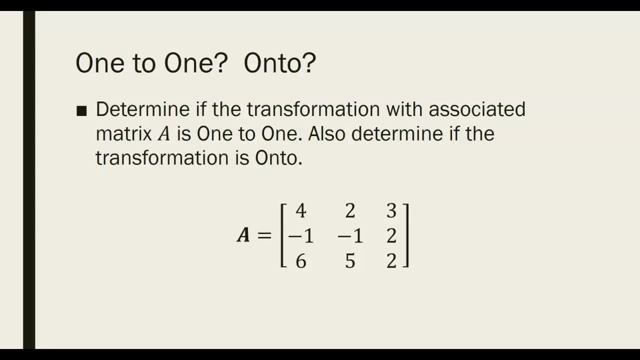 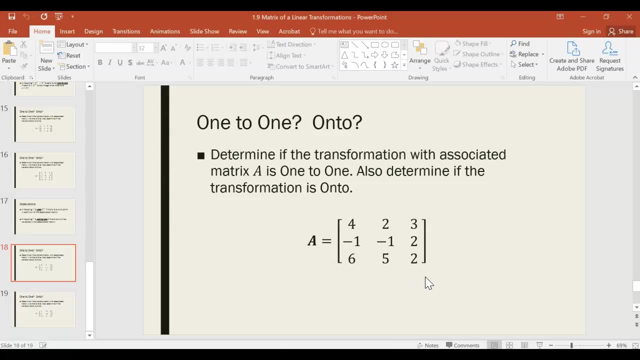 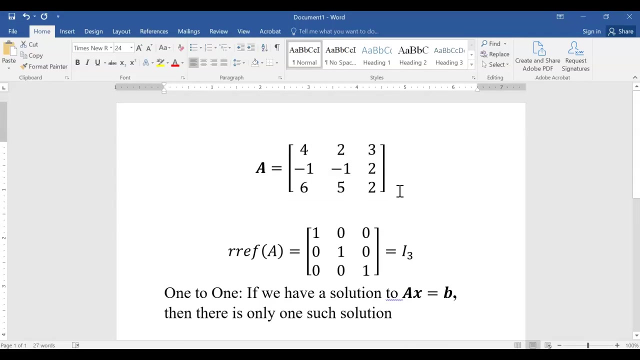 associated matrix is onto or one-to-one. So go ahead and push, pause, Pause on the video and do that. There we go. So here's what we go, Here's what we did, I'm sorry. So we take this matrix and 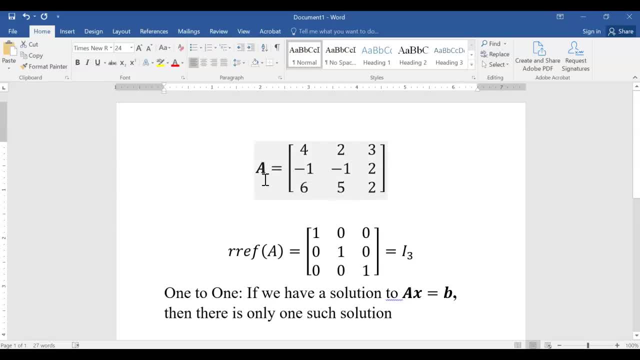 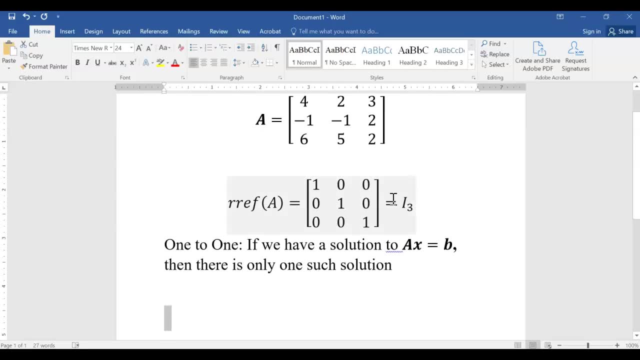 basically we're thinking matrix equation, So we put that in row-reduced-sessional-on-form. Now, if you do that for this matrix, you get the 3x3 identity matrix. So I3 is what we would call, that I sub 3.. And notice: we can ask. 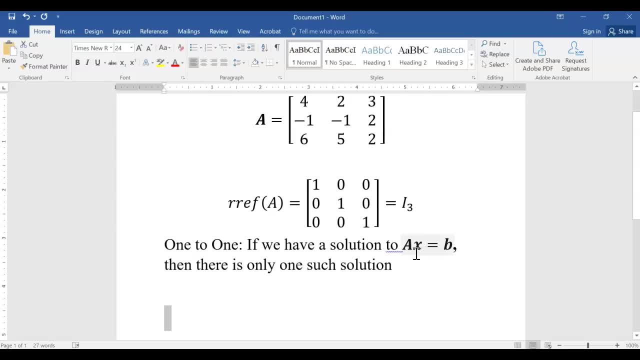 is it one-to-one? All right, If you have a solution, there's only one such solution. So if we have a augmented matrix here, are there any free variables? Is there any situation in which we can get an infinitely many solutions And the answer? 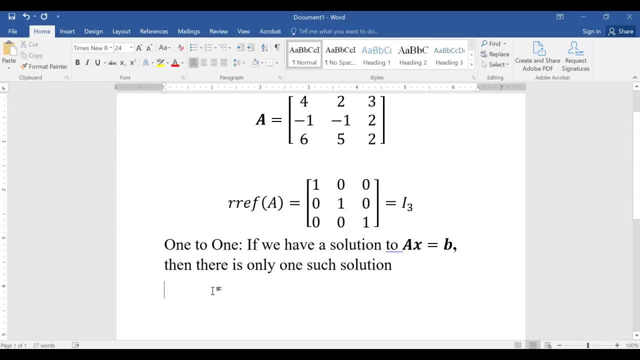 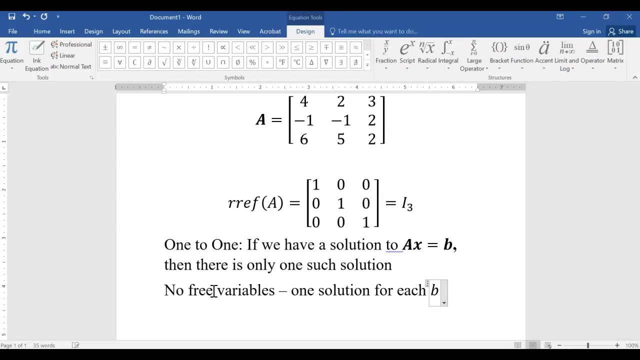 is no. There's no free variable columns, no free variables. So, since it's no free variables, there's only one such solution. One solution for at most for each B. All right, One solution for each B means that this transformation is free. 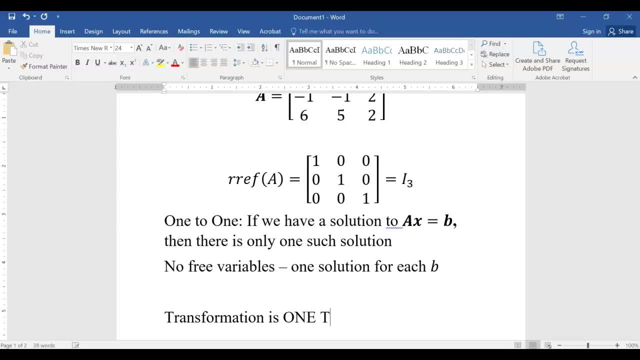 One-to-one. Okay, So we, this one is one-to-one. All right, Let me do that that way. Now, how about onto? So again, remember what onto means. We need a solution for every B we choose, So we're. 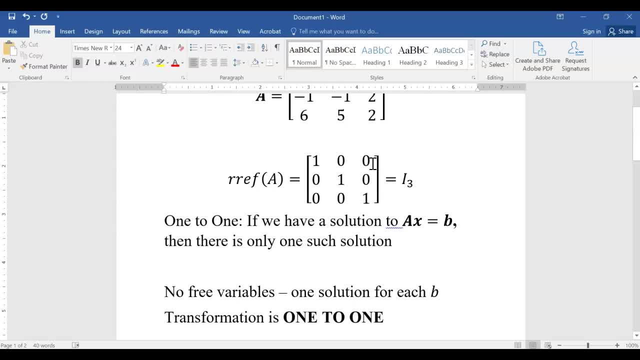 asking ourselves: is there any way that we could get a no solution? The answer is no, because we have a pivot point in each row. So whatever we do over here in the augmented matrix on the right-hand column, we're going to get. x1 equals some. 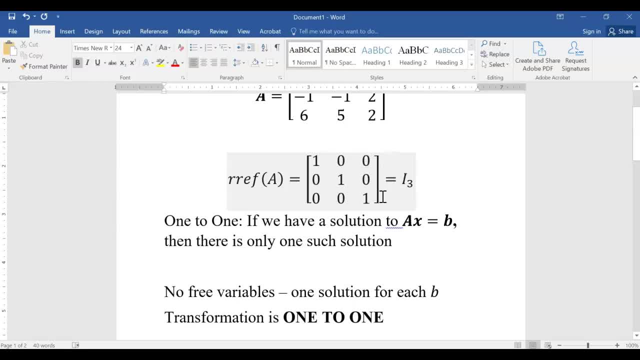 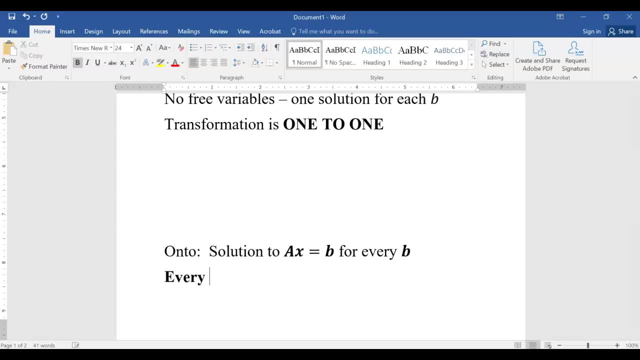 number. x2 equals some number, x3 equals some number, And so there is no way to get a, no solution. So every vector B has a solution And therefore this transformation is onto All right. So every vector has a solution. 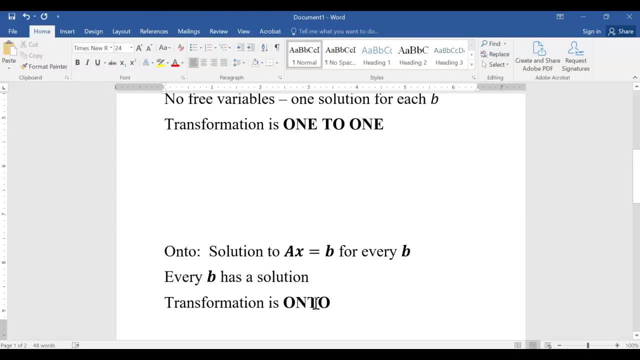 And therefore this is onto Notice that again this in our previous two examples we had like a one was a one-to-one and the other and the onto was not, And the other way it was not one-to-one but it. 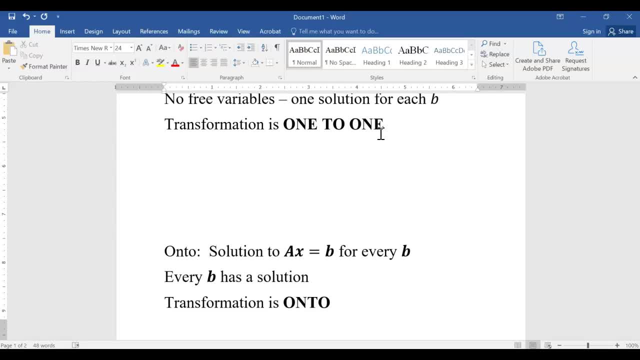 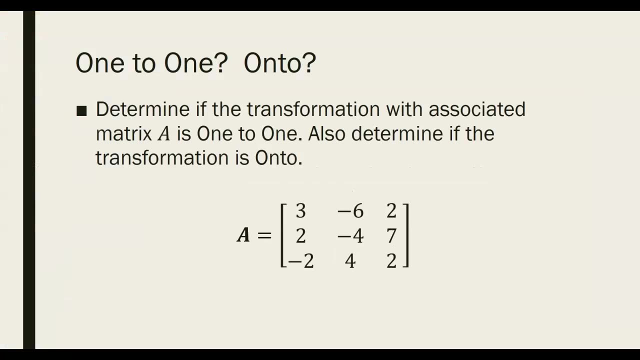 was onto. In this case, we have a situation where our matrix is both one-to-one and onto. All right, I want you to do one more example of that. I want you to take this matrix and see if this one is one-to-one and then 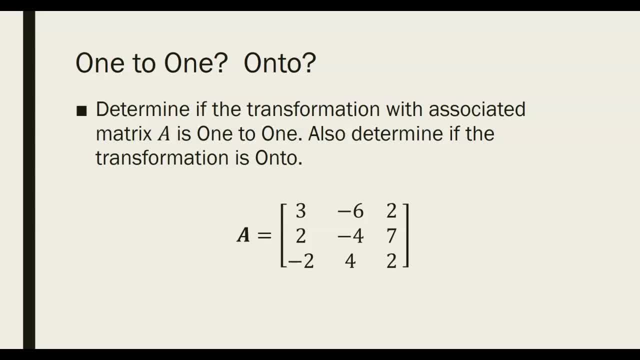 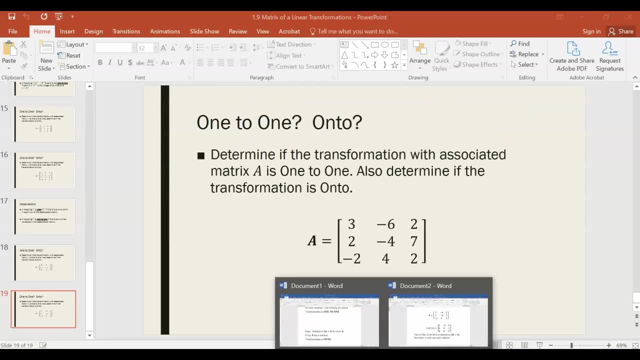 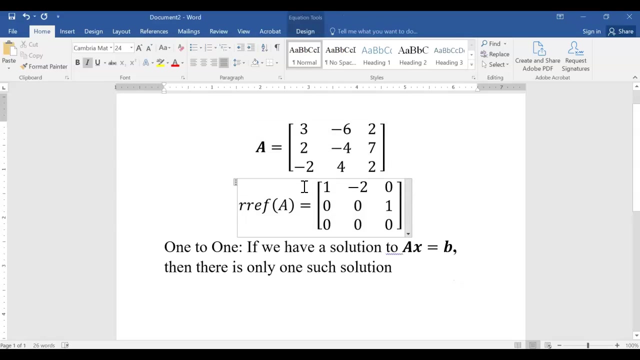 also see if this one is onto. Push pause on the video. All right, So here's what we do. Put the matrix in your calculator, this matrix A, put that in row reduced echelon form. What you get is 1, negative. 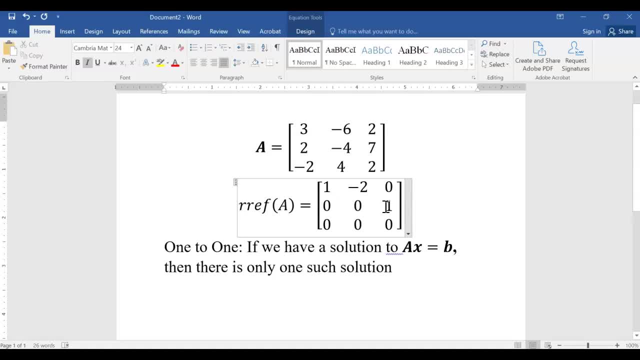 2, 0 in the first row, 0, 0 in one in the second row, All zeros in the third row. okay Now, first off, let's talk about one- to-one. Could this be one-to-one? 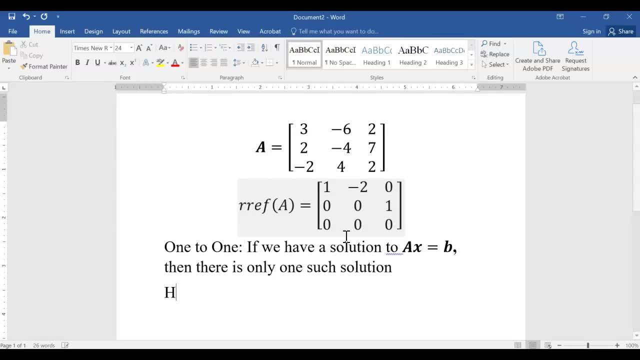 The answer is no. This is not one-to-one. We have a free variable, So there is going to be an infinitely many solutions situation if we can solve for b, So we have a free variable, or this matrix has a free variable. 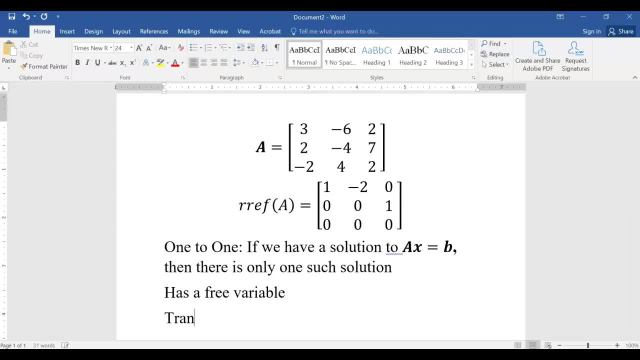 and therefore this transformation is not one-to-one. So this transformation is not one-to-one because we could find a free variable. One-to-one means there's only one solution for every solvable equation. This free variable says there's infinitely many solutions. sometimes, when I solve the equation, 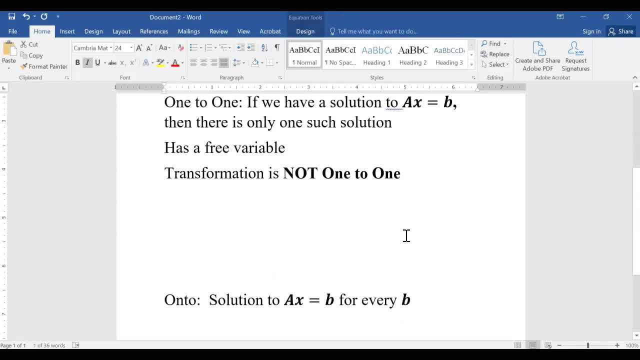 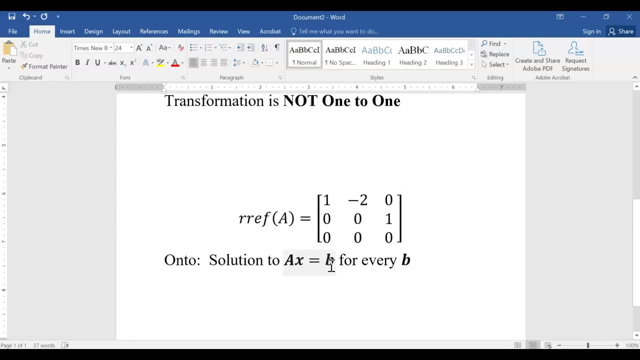 Now let me copy and paste that so I don't have to scroll up again. Let's look at onto. Onto means I can get a solution for every b I choose. Basically, this last row says that we get on all zeros.